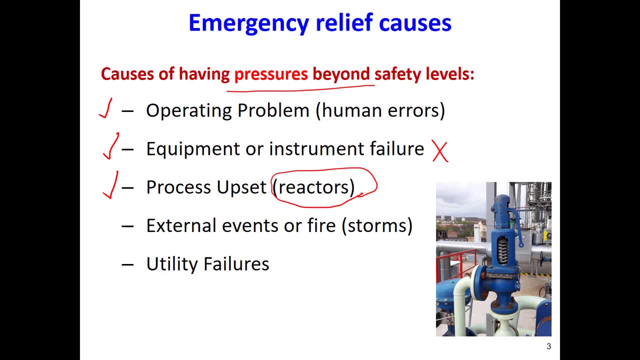 temperature will increase and the same time pressure will also increase. so this is called the process offset. so this can also increase the pressure in the reactor- or external event or fire- let's say there is a fire somewhere in the process or there is a stormy weather that it will destroy, or 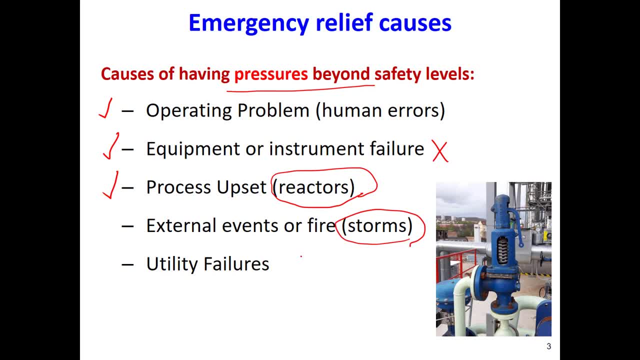 damage one piece of equipment and then that that equipment catch fire. so those are utility failures. let's say, one valve fails, one pressure meter where phase one level meter left. so those are the cases that we might have some over pressure or higher pressure than what is expected. 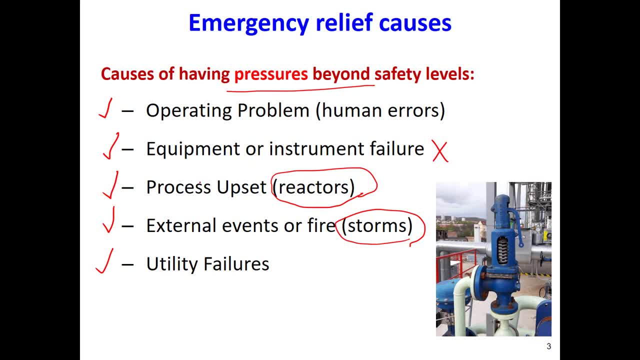 in, like in in the process or in the equipment that we have to find a way and relieve, relieve this, this pressure that we usually use: relief devices, relief valves like dark valves, like one you what you see here. i think, or i believe, in po1150 you should have seen this type of the valve because 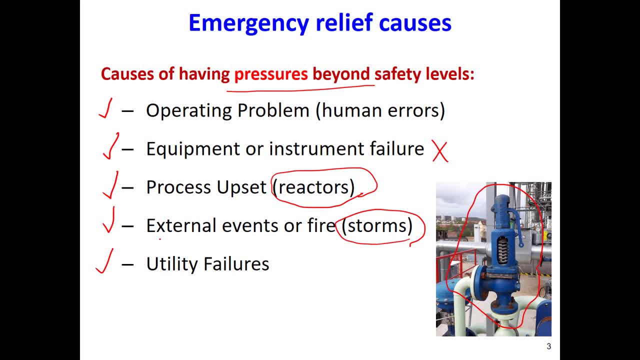 of that, and i believe you should have seen this type of the valve because of that, and so that's One of the topics that we will cover in PO1150 is relief devices or relief valves. So it's such a valve that I'm going to explain a little bit about this type of, in general, relief device or relief valves. 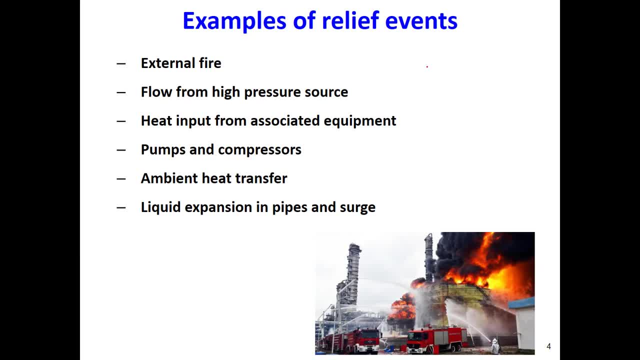 So okay, in which case we need a relief event. Relief event means relieving the pressure. We need to just discharge or purge the pressure from the system. As I said, external fire if you have a flow from high pressure source. 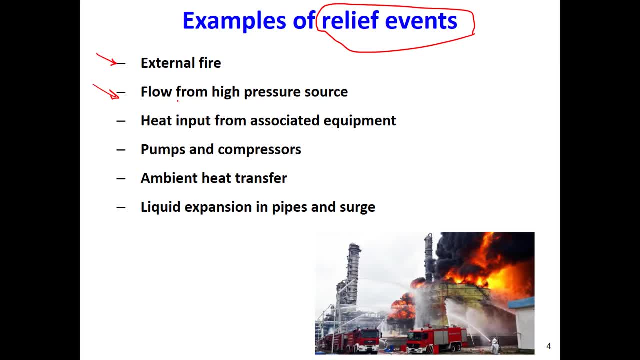 let's say you have a high pressure tank or a column that is working at high pressure, there might be some heat input to a piece of equipment. Let's say you have a tank, you have a storage tank. For any reason there will be an increase in the temperature of that tank or there will be one heat input to that. 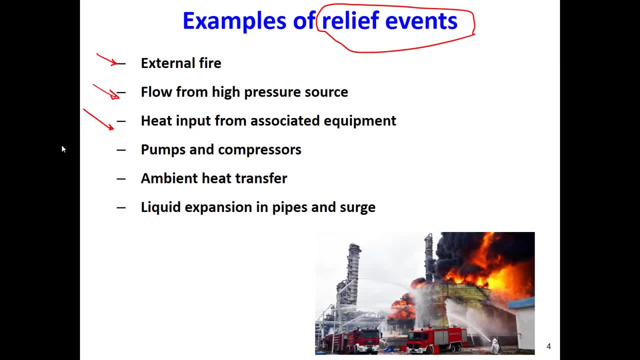 You know, let's say the heater of that tank or the cooling system of that tank fails, So the heat will be added or there will be an increase in temperature. that usually increasing in temperature also increase the pressure, Because increasing in temperature can vaporize the liquid and make more vapor, increase the pressure. or for the gas, we know that PV is NRT. 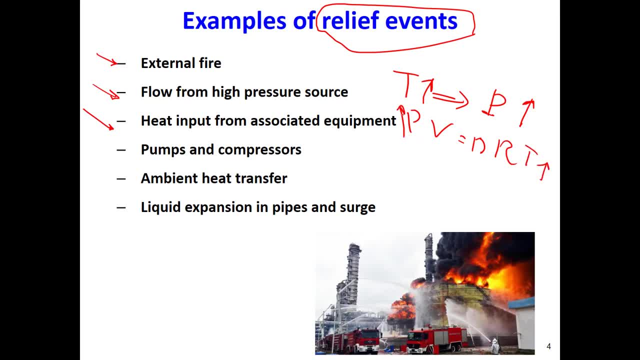 If temperature is increased, pressure will also increase. Pumps and compressors: those are equipment Equipments That the pumps increase the pressure of liquid, compressor increases the pressure of gas. So those are the equipment that we might we have change of pressure. 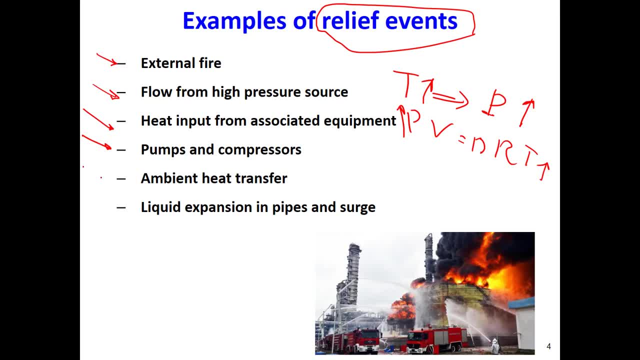 So we have to control them accurately. Ambient heat transfer: So let's say in the summer days, especially here, that temperature goes up, So the equipment they catch more heat than you know, like winter time or let's say at night. 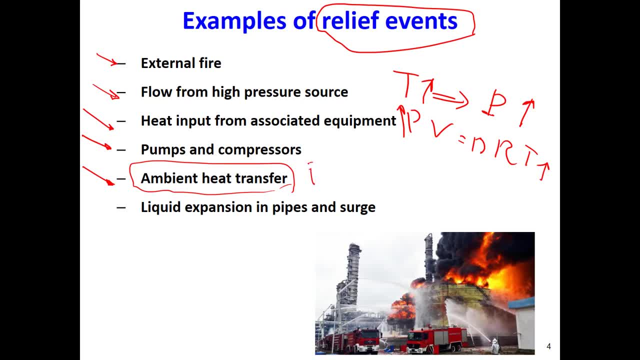 So those are The cases that we can. we might have some increase in pressure and we have to relieve it. Liquid expansion in the pipes or surge tank also is a case that we can have is also cases that we can have increase in the pressure. 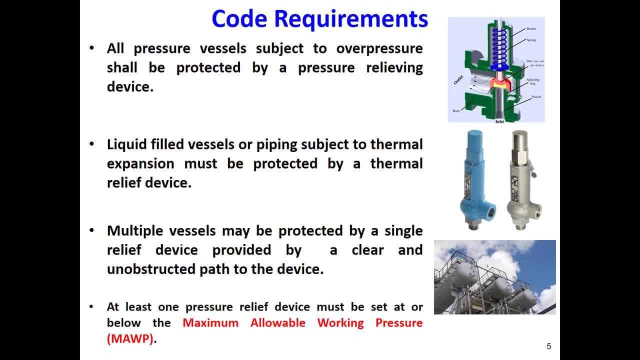 Then code requirements. Okay, So this relief devices or relief valves in general, they have kind of design, Okay. So we have to consider what will be the possible scenario that we need this kind of valve, what are the possible scenarios that we might have some excess pressure in the system and how much will be in worst case? how much will be that expression excess pressure that we have to relieve it, right? 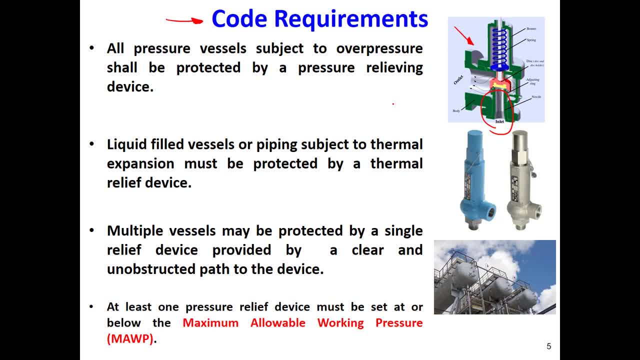 So, based on all this information that we have, we have to go choose and pick the right relief valve. Okay, And there is in some of the slides. I will explain: If you don't pick the right equipment, what will happen to? what will happen to the process or to the devices? 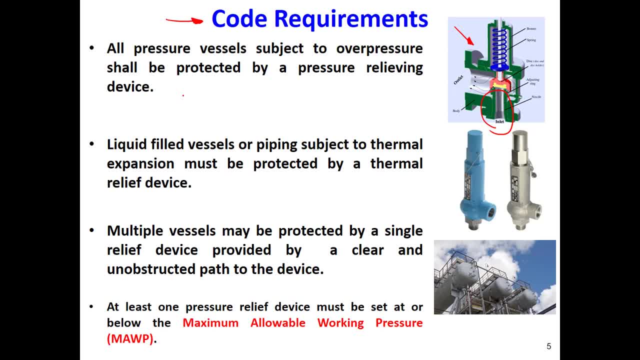 So, first of all, all the pressure vessels, whatever pressure vessels or pressure tank that we have, we that we know that the pressure is high and pressure will also increase, We need to design such a relief valves. Okay, In all equipment, in all piece of equipment that we have high pressure- let's say pressure vessels, pressure tanks, that I already that we already know like which type of tanks they are- we need to have a relief valve. 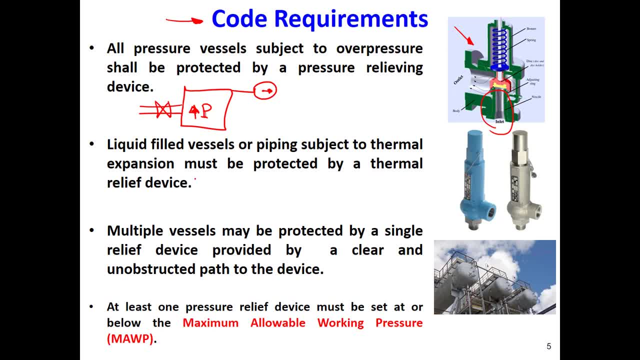 Okay, To protect this vessel, this devices. If you have a vessel which is a a pipe system, piping that is filled with liquid and we we know that that liquid it might goes to a thermal expansion. thermal expansion means that there might be a change in the temperature, increasing in the temperature. okay, there. 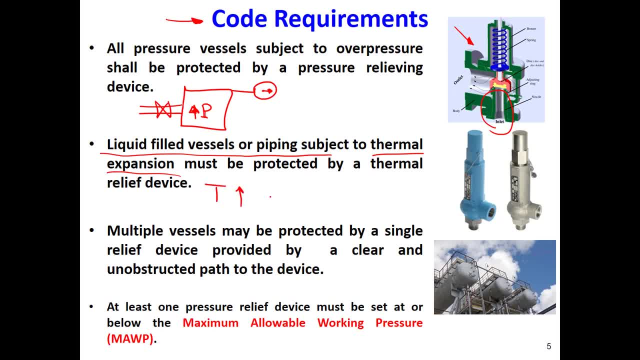 might be an increase in the temperature. that this increase in temperature can lead to increase to okay is a thermal expansion. so there might be some cases that there will be an increase in temperature. this increase in temperature can also increase the volume. okay, thermal expansion for liquid means. 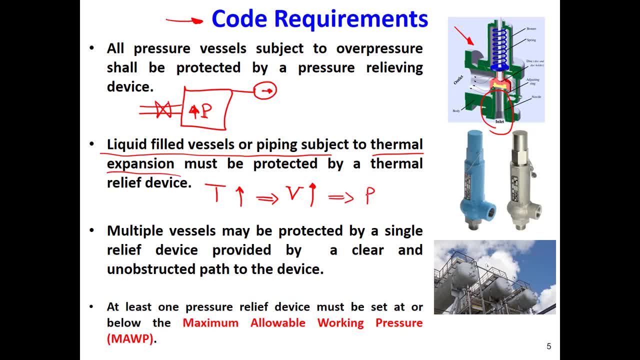 increase in temperature, that this increase of volume, that if it's in the limited space the pressure in that space can also increase. so in that case to protect the device we need also a relieving system like that: multiple vessels- okay, so when we have multiple vessels, or let's say 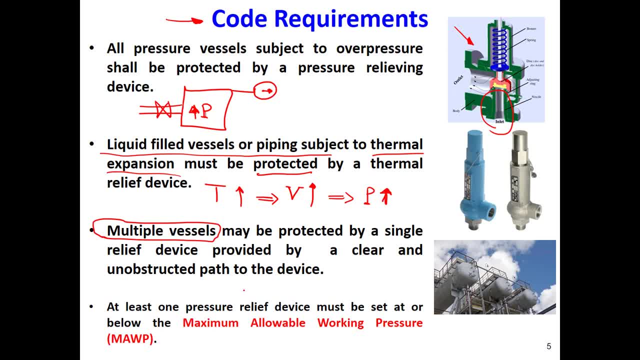 connective system. okay. so when we have multiple vessels? okay, so when we have connected times connected vessel, connected pressure vessels, when we have multiple of them, we can use one single relief device. we don't need to use several. okay, but as long as that we are sure that there is no obstacle or there. 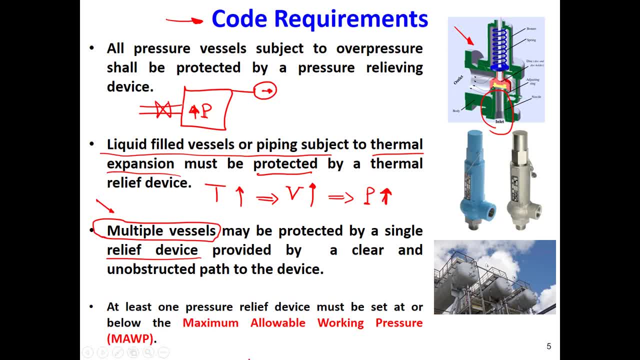 is no, and I mean like there is no issue between the between in the network of this vessel. there isn't like all this wizard are connected. I mean pressure in one vessel'sTrust is goo. that means that if it application properly and if, let's say, there is one in90 increase in pressure in one vessel, that can be. 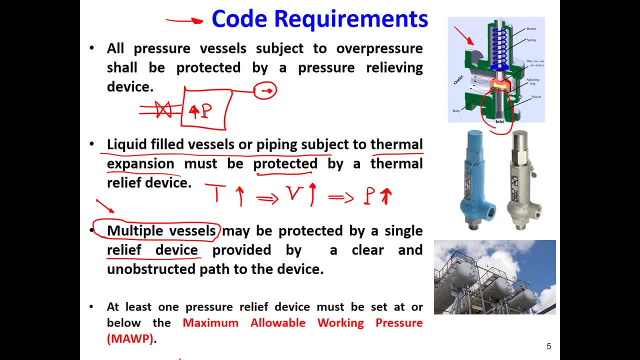 detected, even in the neighboring or in there in the other vessels, then for sure we need to all the time okay, when we have pressure reliefs, okay, purpose will give to us such like such devices. you know, like each of these devices they have that you know they have such a springs here that we can choose the type of this spring, or there is. 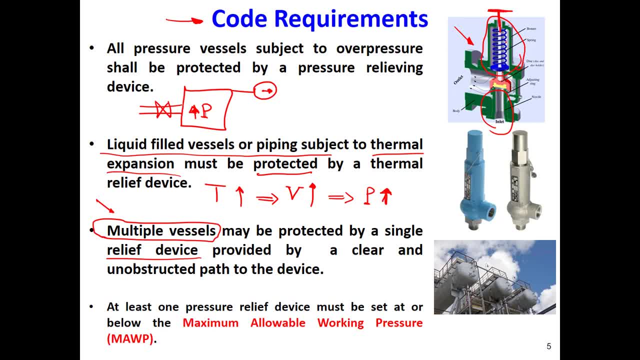 usually a screw here that you can turn this screw and you can change the tension of this spring. and by changing the tension of that spring you can change the pressure that the valve will act. okay, the relief pressure, in which pressure the valve has to be open or closed, you can change it. so 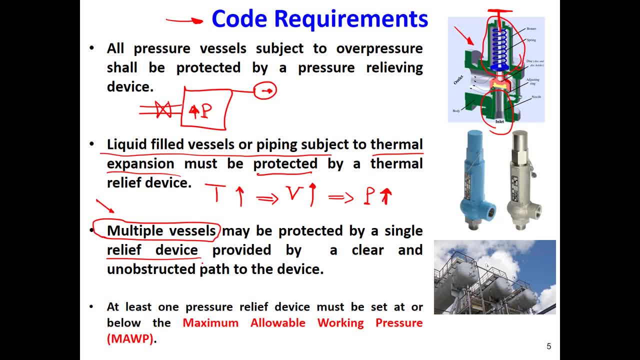 there is also okay, so we have to, and also all the devices that we have. any equipment in the process. it has a parameter that is called mawp- maximum allowable working pressure- which is the maximum pressure that is allowed to reach in that equipment. if we pass this mawp, we can damage. 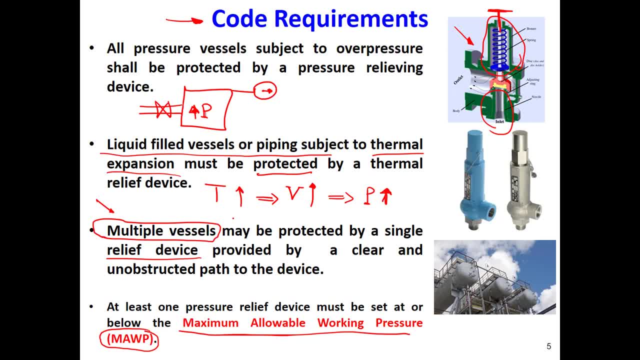 the equipment and we can damage the equipment and we can damage the equipment and we can damage the equipment. okay, we can damage the equipment. or in some cases we might have explosion or we might have, you know, the equipment might burst. so we always set the relief device. okay, we always set. 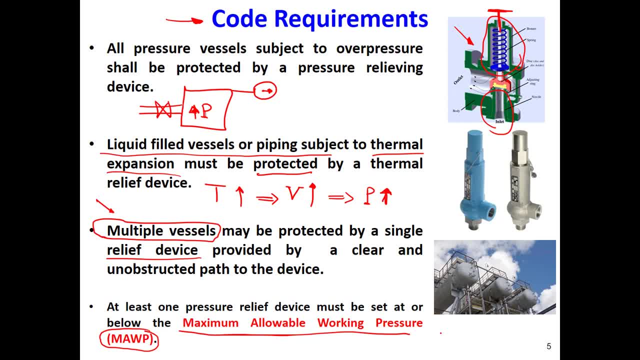 the relief device below, below, below this. most of the time we we we adjust, we set the relief device below below this most of the time we we adjust, we set the relief valve below the maximum allowable pressure in this situation and if it doesn't allow the pressure to increase, Okay. 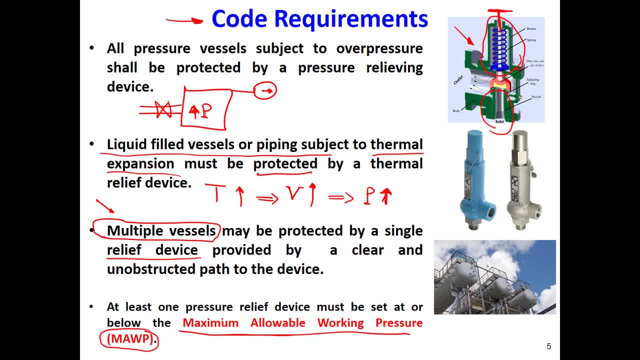 there is matter of doing this in this situation, although in the case of use of this machine, Fighting can be handful and I have opened 4 drives of some kind of certified Ag vergessen which I have seen the enemies ofunted used to start such drives when it was running on. Okay, is the maximumapan working pressure. okay, is far from the pressure that that equipment might burst or explode. Okay, this pressure maximum atята Bőmer, working or operating pressure is usually far from the pressure that will lead to explosion or, you know, not like two, two to the. 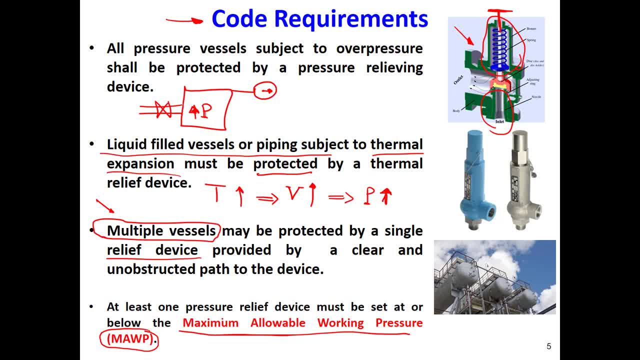 burst of of the equipment. and the reason is that you know, like this is for safety, like we want to be defined, this pressure for the user, for the operator, to make sure that he's all the time working under or, you know, very close under or, in the worst case, close to this pressure and he doesn't pass it if he passes that. 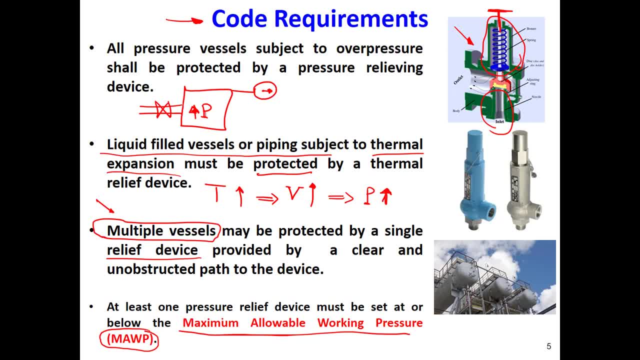 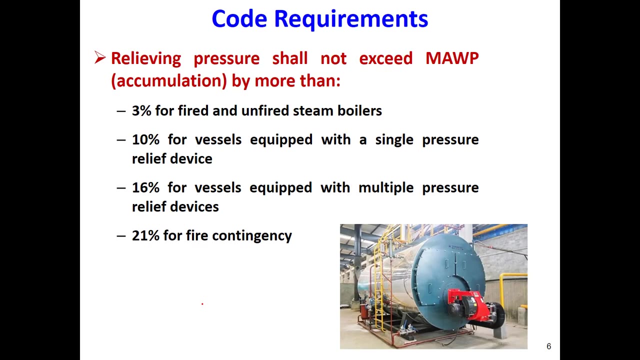 is a, you know, like he has to, like he has to receive a warning that he's passed the MAWP, the maximum allowable working pressure, and we usually set this valves in this pressure or below it. okay, so if the pressure reached in the vessel reach to this pressure, the valve will be open. then okay then, in general, as I said, 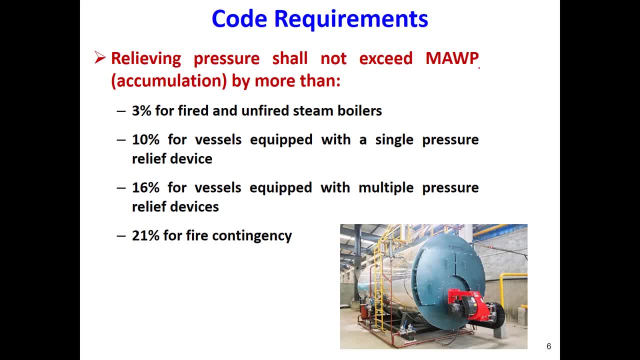 okay to be, to make a sure, to make sure that we're not the valve, the relief valve is not going to be open, I mean unnecessarily. I mean to make sure that the valve it doesn't open or it doesn't take action. that is not really critical case. so, as I said, it's. 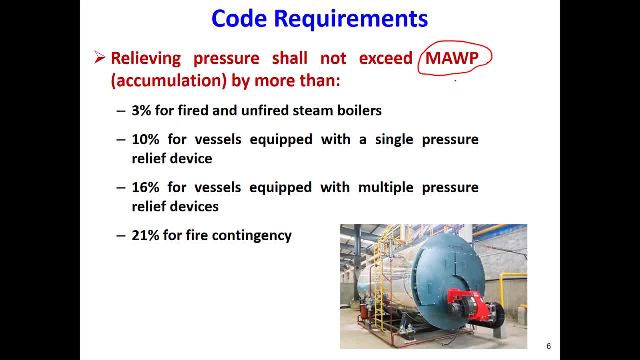 better to have all the pressure valves, the relief valves, to to work at this point or below it. but in some cases we can set the relief valve, the relief pressure, the pressure that the valve will be open, a little bit above this pressure as well. okay, because we, because 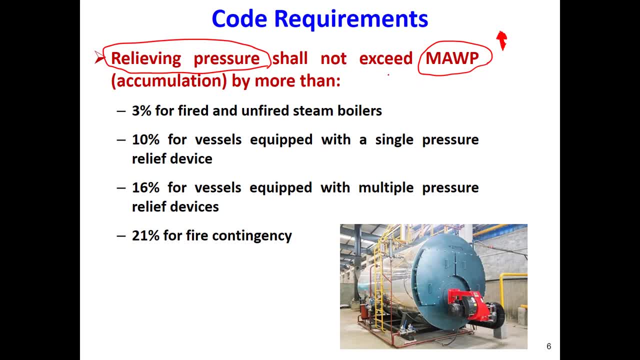 as I said, the maximum operating pressure is not the really the pressure that we might have exploded. so we can. he can adjust the relief pressure, the relief valve, at a pressure a little bit above it to make sure that the valve it doesnt open unnecessarily. so there are some, you know. it's common that in the process the 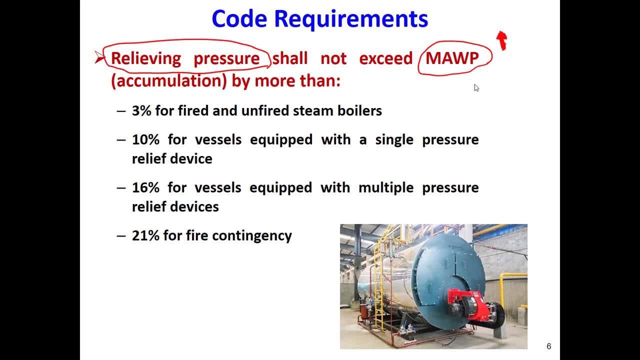 vessel goes a little bit above the allowable working pressure, but it's not still dangerous. you know we don't want that. as soon as the equipment reach to this pressure the valve start opening. you know we can give it a little bit more room. so for for, for example. there are some cases here, for example for the 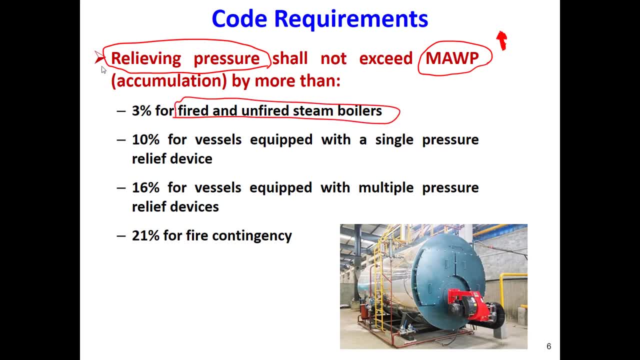 fire or on fire steam boiler, we can set the relieving pressure like three percent more than the maw mawp, a little bit three percent more than the allowable pressure if, if the, let's say, we have vessels like multiple vessels, that has only one single pressure relief device, so which we 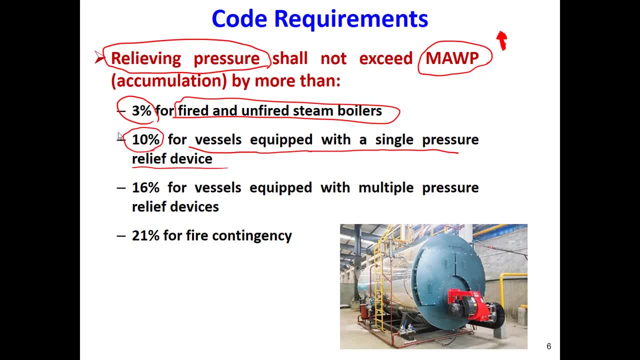 can. we are allowed to set the pressure up to 10% more than this pressure if we have, let's say, multiple vessels, that they have also multiple pressure relief device. so in this case, since we have multiple pressure relief device, we have more freedom, so we can set the operating the relief pressure up to 16% more than. 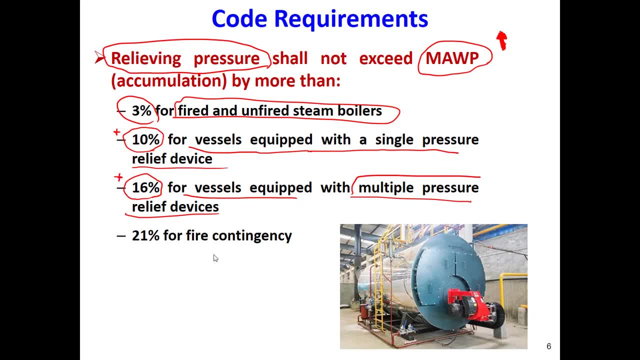 the allowable pressure and in case, if there is- you know, like some, in case there are some you know- possibility for the fire, okay, that in the device, in the process, in the equipment, we can adjust a relief valve up to 20% more than the maximum allowable working pressure. but this is kind of. 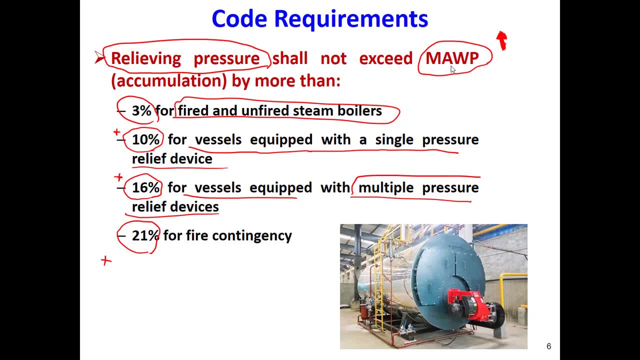 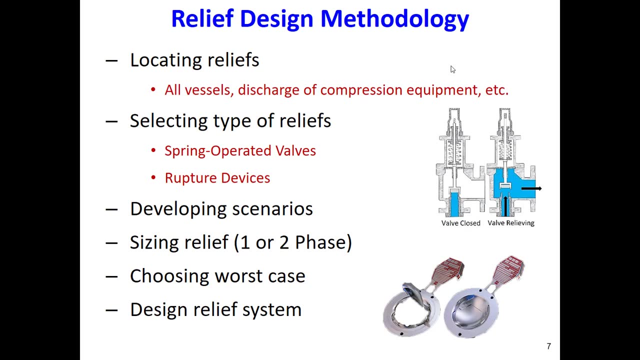 different from what we have seen in the previous video. so this is kind of different from what we have seen in the previous video. so this is kind of general rule. you know it can be. it can change from one equipment to another, from one process to to another. then okay, so how we design such a device, how we 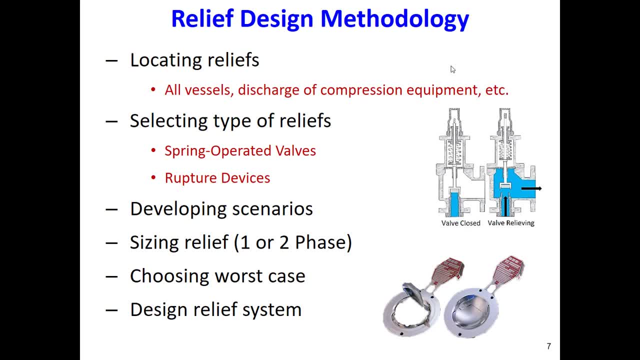 design such a valve relief valve. so first of all, we have okay where we put them all, the vessels, pressure vessels or even vessels that are working a little bit above the atmospheric pressure. we need to have such a valves in the discharge of compressors or compression equipment. 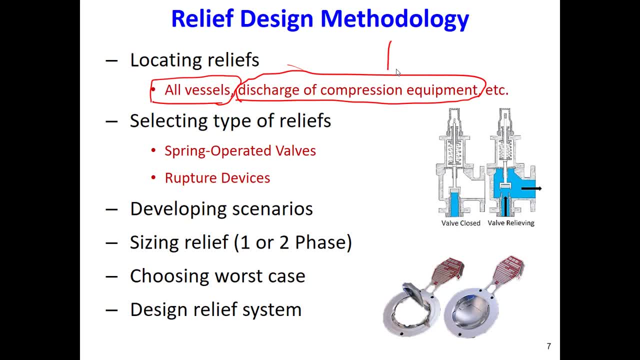 okay, discharge of compressor are usually in a storage tank that that has high pressure, so we can. we should put such a device in in that in the discharge of the compressors and we have, depending to the application, we can use the relief valves or pressure relief valves. 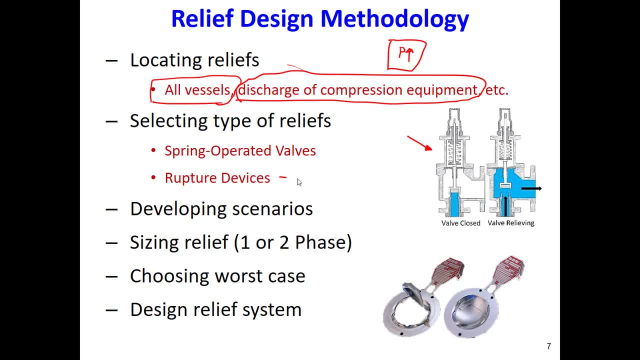 like such a this valve or we can have also rupture devices. rupture devices is a very simple device, is like a metal disc like this disc here. that it's it. it's usually okay, that is, you know, in install on the vessel, on on the pipe that block the vessel, block the pipe and 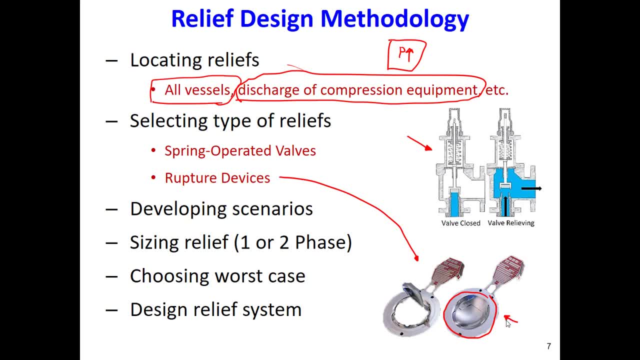 so once the pressure in one side of this rupture, this goes up more than the pressure that is allowed in this rupture. this so the rupture. this will burst rupture and it and it will relieve the depression. in that way it's usually used for liquid service with a very viscous 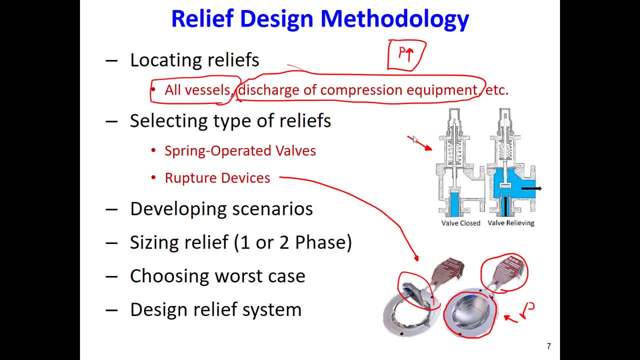 liquid. okay, so like we can use this device or this one, how? okay. then we have to develop scenarios. we have to sit and think about what are the worst cases that can happen. what will be the worst case scenario that we, we will have pressure in that equipment? what will be? 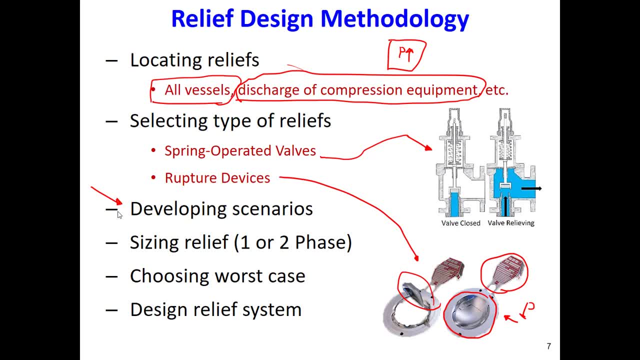 the maximum pressure, maximum flow rate that we need to relief in that equipment. then we will use, we will size the relief. you know we will do. we will use some calculation and find the right size of the relief valve, as I said, choosing the worst, worst-case scenario and also at the 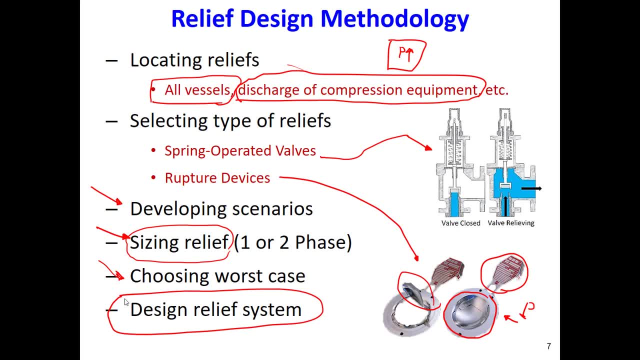 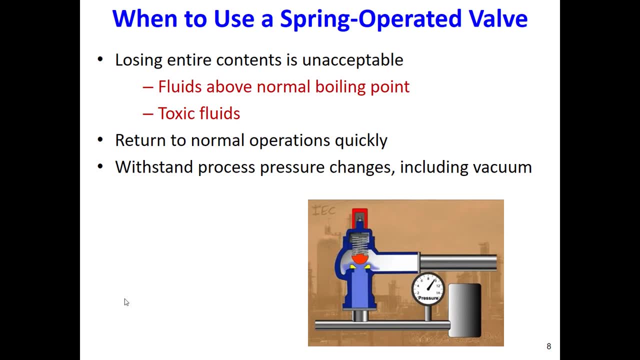 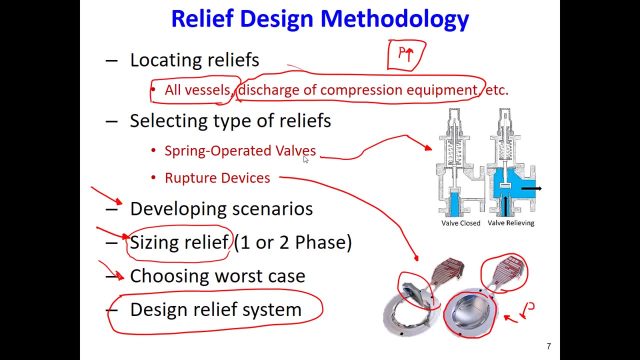 end, we will design the relief system. if we need one relief valve, if we need multiple relief valve, this is what we will design at the end. okay, so, as I said, we can use a spring operated valve or relief valves or rupture devices. okay, so, relief valve, they usually have a spring. 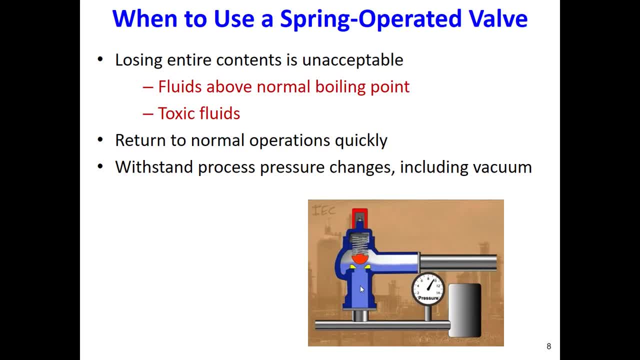 that we call. that's why we call them a spring operator. so here you can see in this animation that I put for you at first that the pressure in the line is not, is not a lot, so this valve is closed. okay, once the pressure in this line increases. so it. 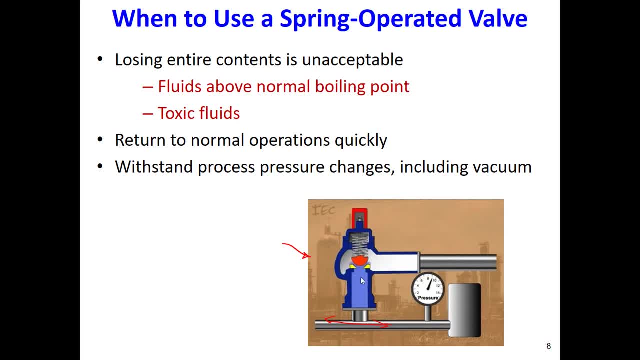 then the fluid, the liquid here, or the gas, will push this, this spring up. you can see, this is a straight leg right and it will. the gate will be open and it will relief some. it will in the pressure and the pressure will increase, increase. so, as I said, we can. there is a stem here, there is a wheel here that we 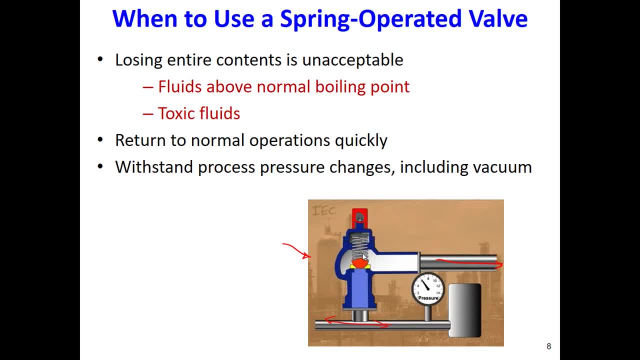 can adjust it, adjust the tension of this spring, and adjusting the tension, it means adjusting the pressure- here in this part so I mean the relieving pressure, so like where we, in which condition we will use it, so when, first of all, when, in the case, we don't want to lose the total content, the entire. 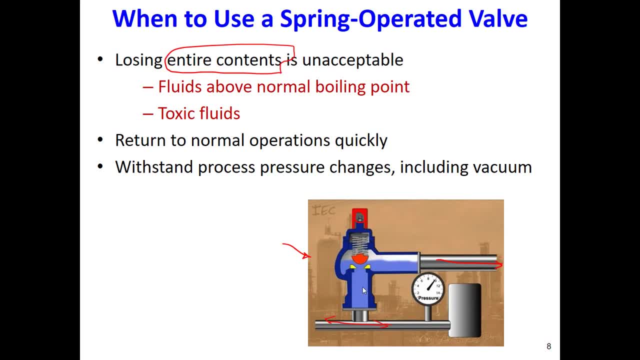 content of the pipeline or the vessel. we don't want to lose, we just want to lose a little bit to adjust the pressure. that's all. when we have liquids, fluids that are operating at the in, that are in in the above the boiling point, when we have toxic liquids that you know, 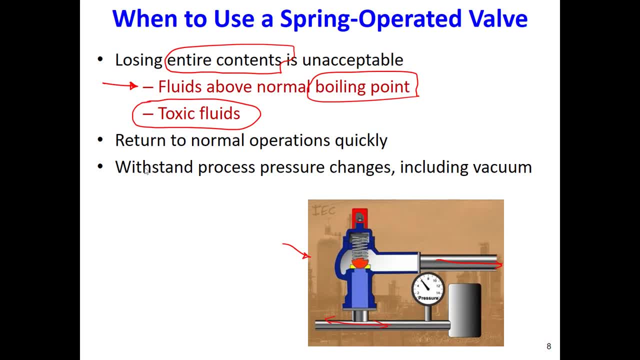 if we relieve all of them, if we lose all of them, so it can be dangerous for the workers, for environment, society, whatever. and then we want to go back to the normal operation quickly. so here the valve will be open only once it is needed, and once the pressure is relief, it comes back to its initial condition and the process. 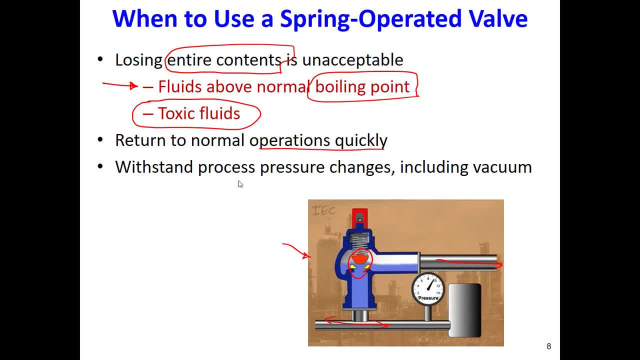 will be working normally okay. so we want a quick action, quick return to the operation, normal, quickly. and this valve can also tolerate the change in the proper process, changing the process pressure. so, as I said, we have such a stem here that we can move it. we can move it clockwise or counterclockwise and by moving that stem 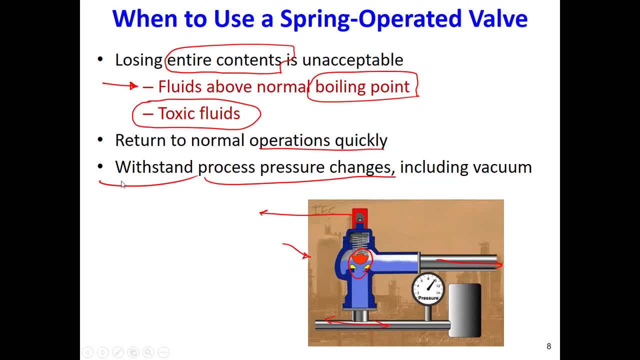 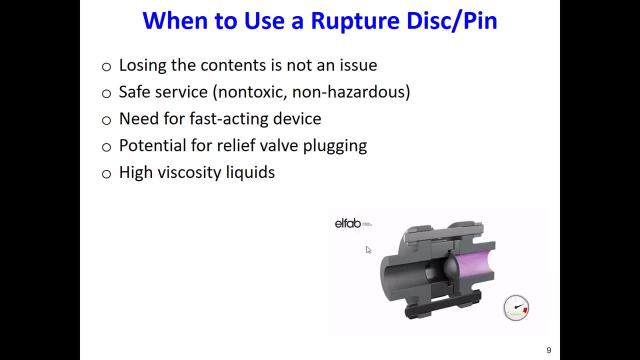 we can adjust the relief pressure. so let's say, if that pipeline is moving tomorrow or next week is working in different pressure, so we can also adjust the relieving pressure here. so it gives us a lot of flexibility, rupture this that you can see here. so once the pressure in the so is like is used in the pipeline. 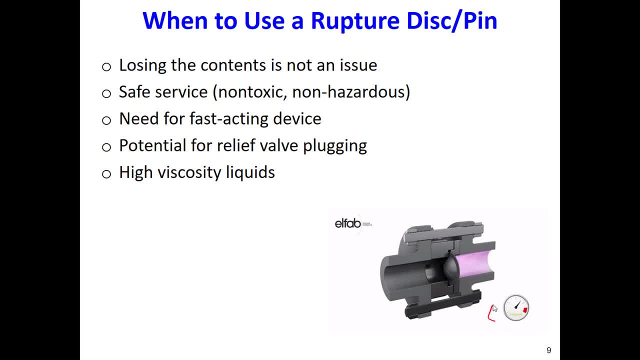 to block the pipeline or vessel and once the pressure increase up to a certain pressure, which is a design, the rupture pressure, so that this will will rub the rupture with the rupture will happen and it will relieve the pressure. so, in which case we will use this type of device first when losing all the 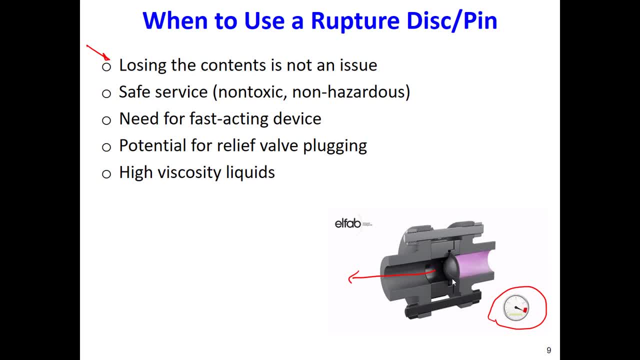 contents is not the issue is acceptable because I, when the rupture happen, it cannot comes back to its initial condition that was blocked or closed, okay, so in that case we might lose all the content or the big amount of material. so if before us there is no issue to lose, it's fine. we can directly change the 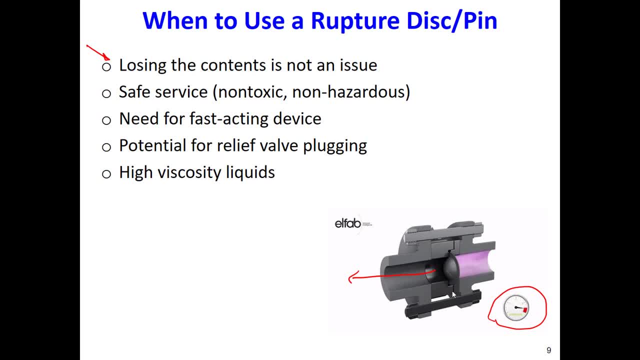 pressure, because you can change the pressure when the Nawab process works on the then, since usually you know we relieve a big amount of materials, so we have to make sure that we install it in a pipeline or the vessel that doesn't have toxic or dangerous material. 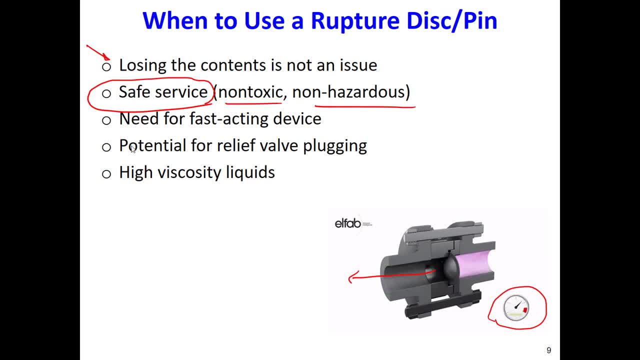 so for safe service or non-toxic or non-hazardous material or streams, it will be used. it's a very fast acting device. it will fast, it will act, i mean quickly as long as, as soon as pressure reach to a rupture, pressure it will rub. and in case if we have plugging, in case if we have. 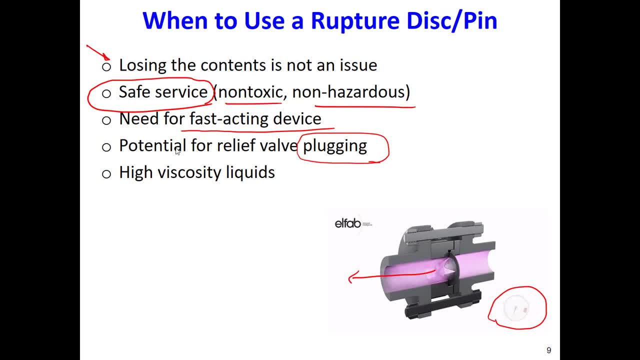 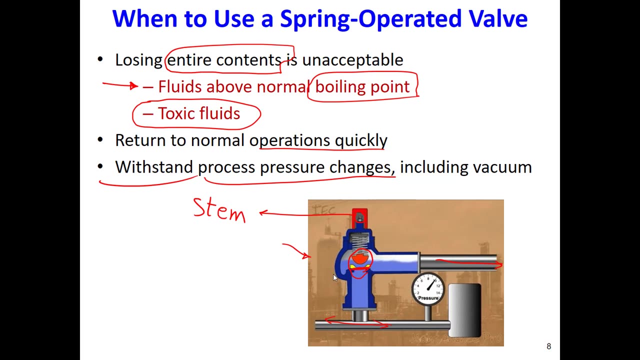 in if in case, if we might have plugging in the relief valve in the pressure relief valve, we will use this kind of device. so pressure relief valve has an opening. pressure, really well, has an opening. if this opening is blocked or you know, with some solid particles or corrosion or for whatever and like that will affect the operation of this valve. 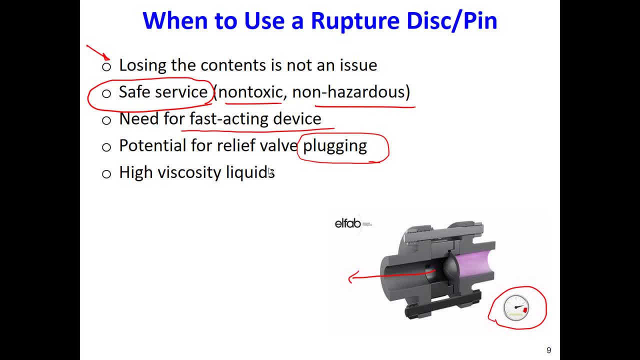 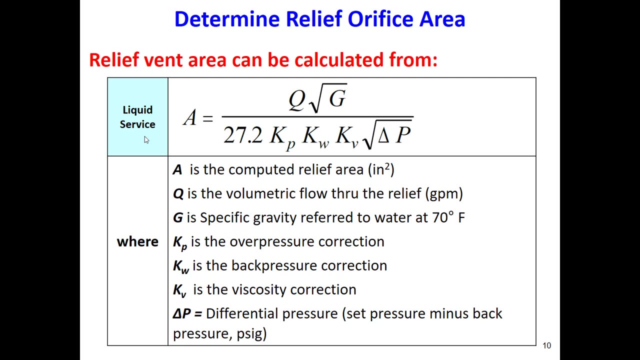 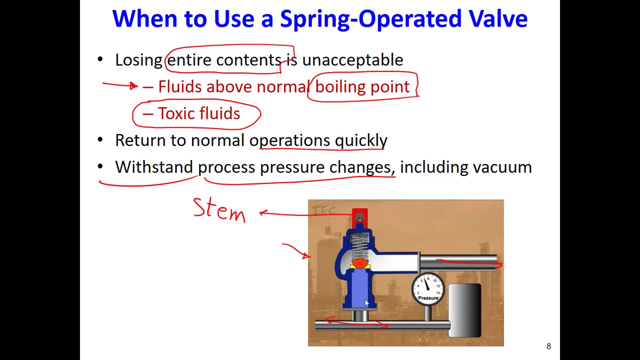 so we prefer to use such a devices and for high viscosity liquids this valves are also more prefer then making that you know, in case you done, even in high viscosity those typeだから it is okay. there are some equations. so what we have to do for for the relief orifice area. 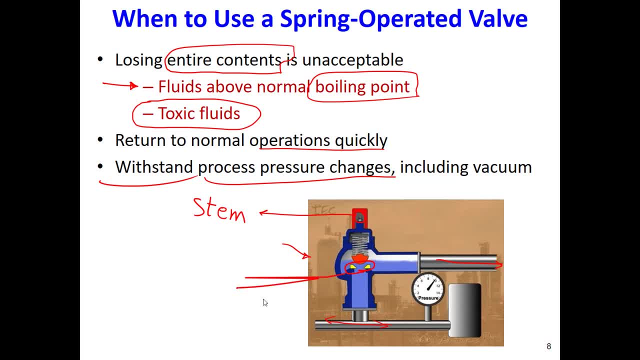 i mean here, this area here, let me okay, for the relief orifice, the area here. so we need, we need to do some calculation. okay, one of the when we are talking about sizing the relief system and relief valve, one of the main important parameter is this area, the place which is located in the middle here. 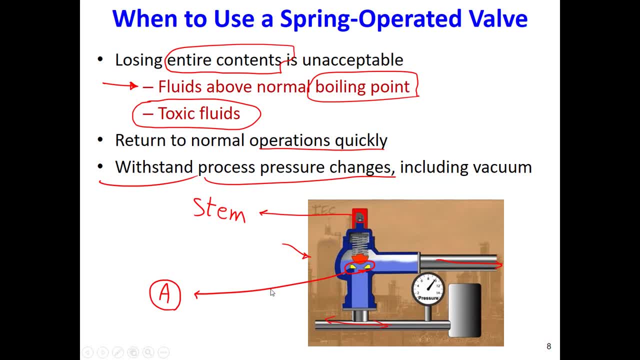 area, the area of that orifice or the reliefing areas. that depends to the capacity, the maximum capacity of the air or the gas or liquid that that is going to be to go through that, through that orifice, and also some other parameters like pressure, temperature, you know, density. 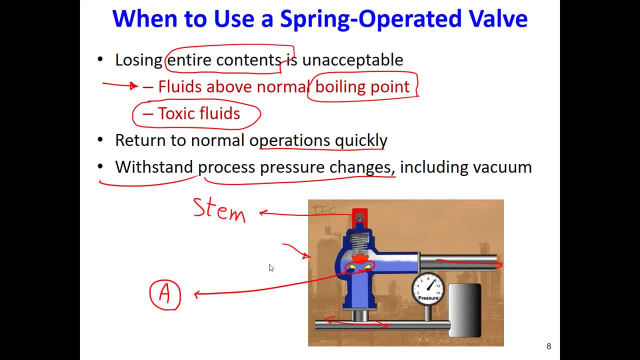 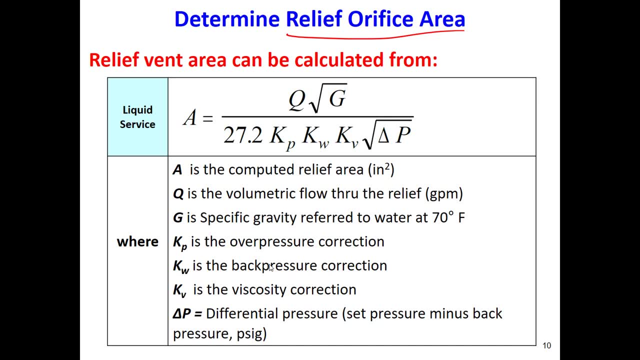 and some other operating parameters. there are few equations that can be used to to calculate that area, that I'm gonna just show them to you. so first, okay, first of all, for each system, either liquid gas or vapors or steam, we have different equation for liquid service. this is the equation: 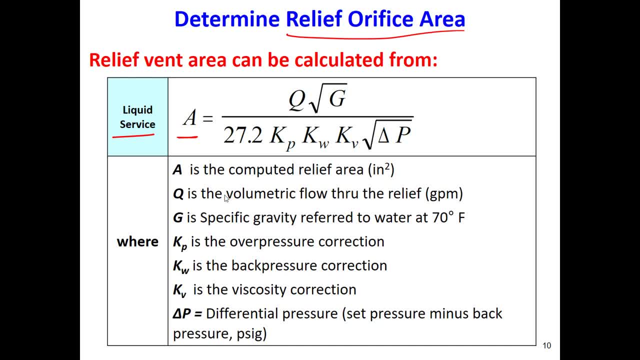 that is being used by most of the engineers. a is the area, Q is a volumetric flow rate, G is a gravity, KP, KW, KV. those are all some factors, some correction factors that will be given to you and is available in the handbooks, in many you know, like valve manuals, handbooks and differential pressure, which is the pressure like. 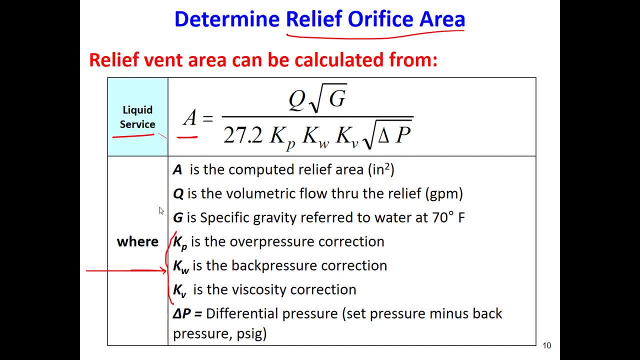 before and after. I mean the set pressure of the valve and back pressure. okay, so if the valve is is connected to the vessel, so is the back. is the pressure that is set here? okay, the set pressure, the set pressure, the set pressure and the pressure here. delta P is the difference between the set. 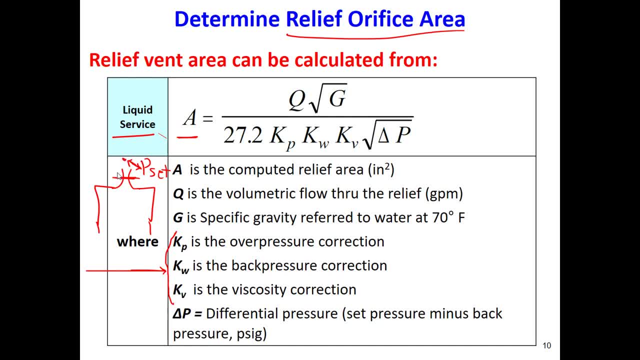 pressure of the valve and at atmospheric pressure this vessel. it might be connected to another blown up, laugh whistle. you are seeing, though, that is cuma. So the pressure is not necessarily atmospheric. The exit of the pressure relief valve might be connected to another equipment or to another place that doesn't have necessarily atmospheric pressure. 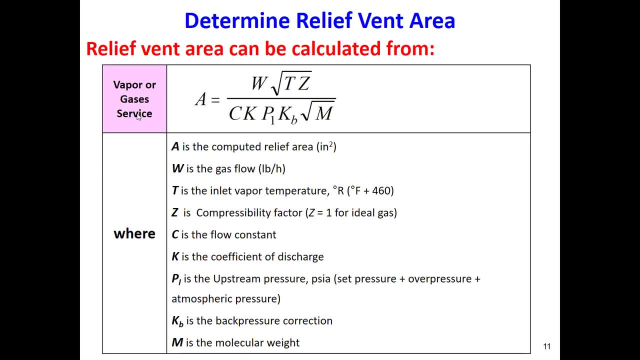 This is for liquid service, For gas services, vapors or gas services like, not vapor, I mean like all the vapor except the water vapor or steam. we will have such an equation that again we have W, which is the gas flow rate, T, temperature, Z, compressibility factor, C, K. 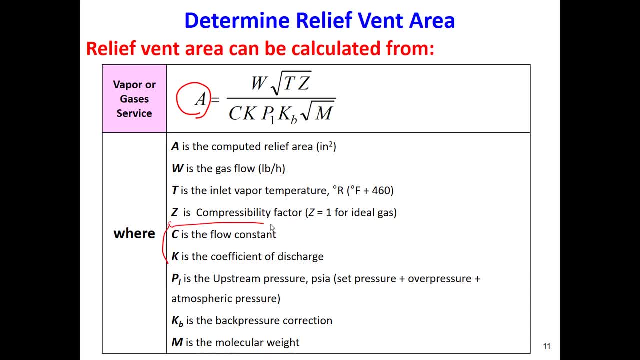 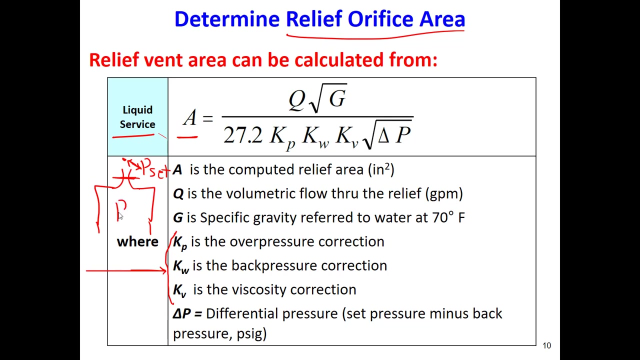 Those are some factors that will be given to you. It's available on the okay, even KB. Those are some factors that you need to use. M is molecular weight. P is also the upstream pressure, the pressure before the valve. I mean the pressure if the valve is connected to a vessel, the pressure of this vessel. 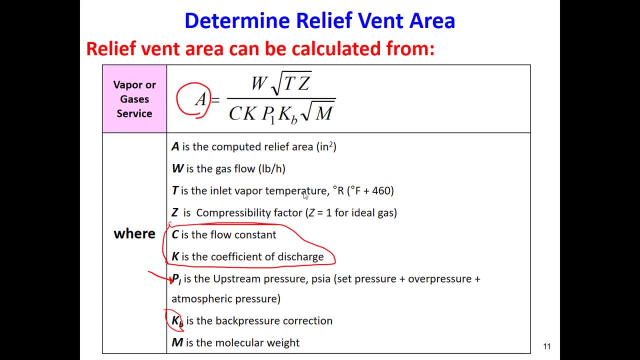 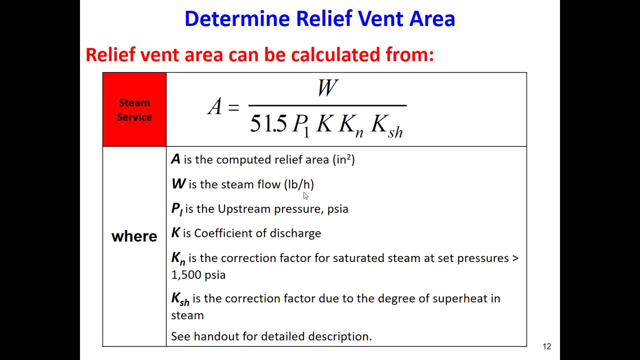 I mean it can be set pressure plus overpressure and atmospheric pressure as well. Then okay, for the steam systems, steam services, we will use this equation Again: W is the flow rate, PI is the pressure, K, KN, KC. 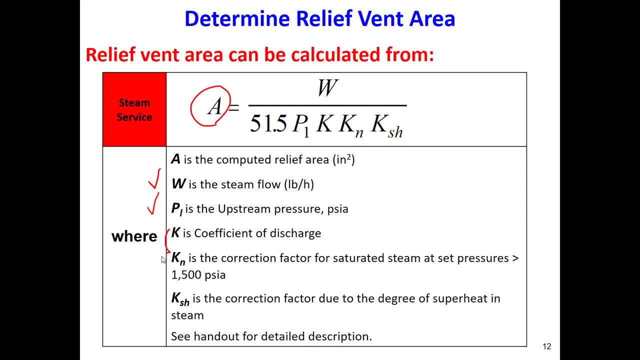 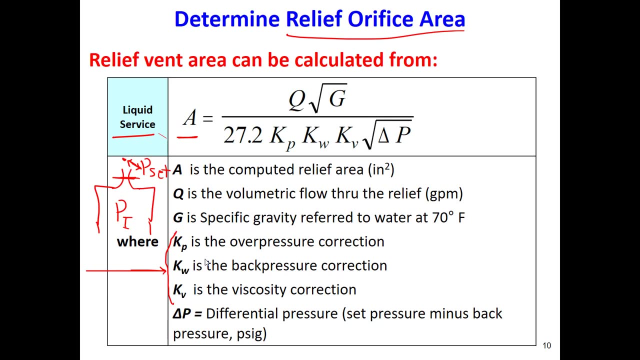 KH, KSH. those are some again, some factors that will be given to you most of the time And, yeah, as you see, like most of them, they are very simple equations. You just need a few parameters You can put there and find the diameter of the orifice or the reliefing section. 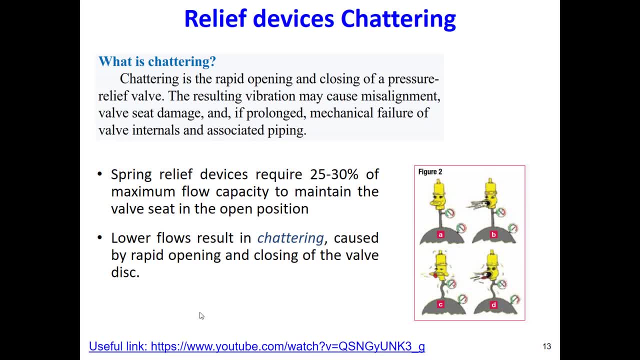 Okay, Chattering So like, I put one YouTube video for you here. Please watch it. This presentation is also available on D2L, so you can download it and copy this link on your browser So you don't need to type it all here, like as you can see here, because sometimes it's difficult. 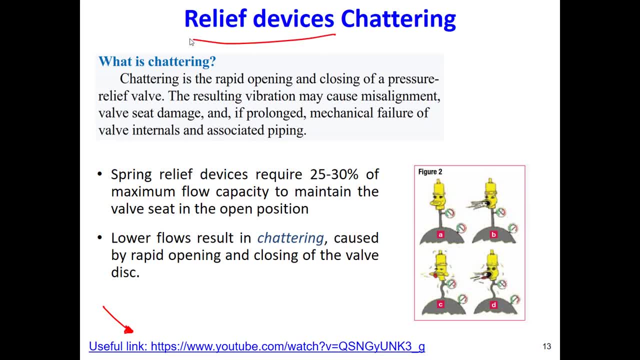 So chattering is an issue in relief devices. Chattering is chattering, or we can call it. Chattering is when the valve starts singing. okay, When the valve starts singing- And you see this figure here- It shows what will happen to the valve. 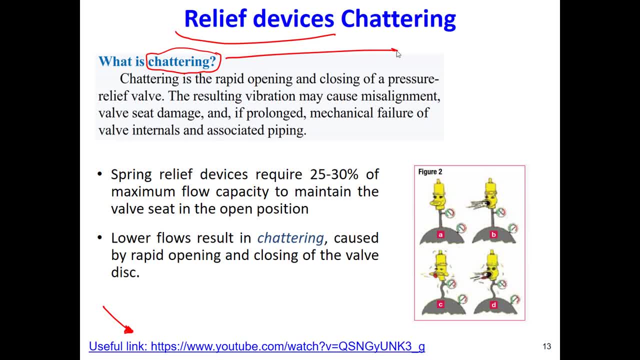 So chattering is when we choose a wrong valve for that process or for that vessel or that equipment, When we choose a valve that is not fit to that pressure, to that flow rate and to that equipment. So it's when 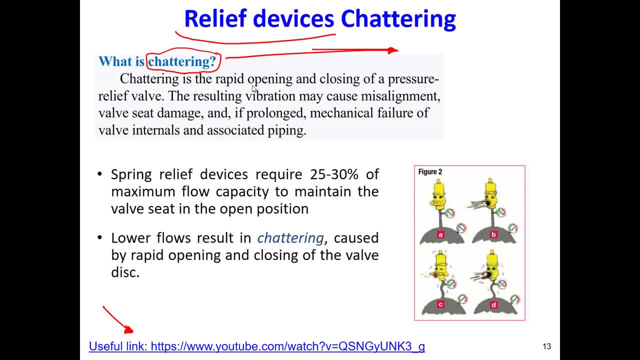 It's when the valve will be open and close rapidly. There will be a continuous opening and closing of the valve that will make a noise like a chattering noise. And since the valve will be open and close rapidly- okay, will be open and close rapidly- it can damage you know, like it can lead to misalignment. 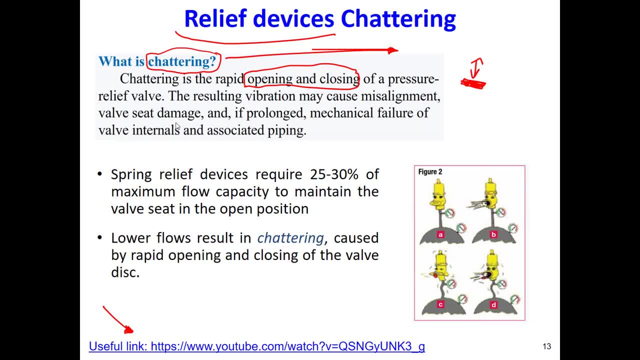 It's like it can create a big vibration, It can damage the seat, the valve seat And, if you know, if it continues, it will be associated with some mechanical failures of internals of the valve and even the piping system. okay, 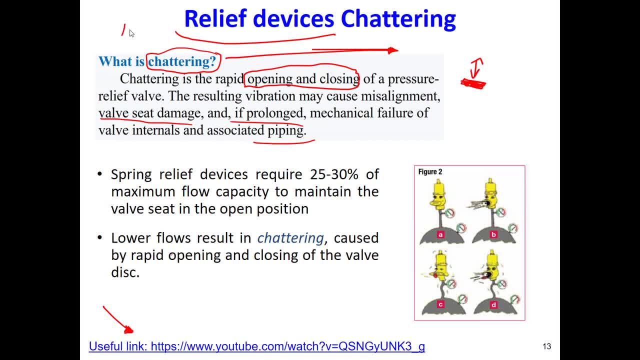 So it's an issue in the relieving system. So this is why it's important. Please try to learn it in details And usually okay, Okay, usually let's say if, if you, once you are sizing the valve, you will find the maximum, you will find the maximum capacity of the valve. 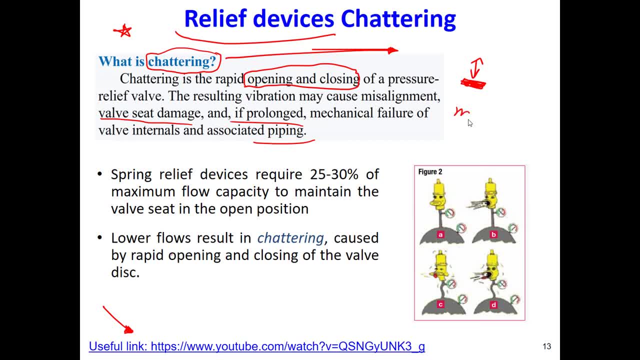 You will, I mean you calculate the valve based on the maximum capacity, which is, let's say, the flow rate of 100 kilogram per hour. You will, I mean you calculate the valve based on the maximum capacity, which is, let's say, the flow rate of 100 kilogram per hour. 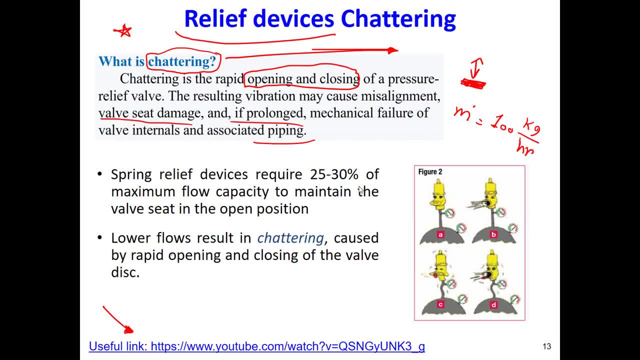 Just just imagine like this: So usually we need 25.. So you design your valve based on this maximum capacity. Your valve has to be able to allow this much fluid if it's open: 100 kilogram maximum. this much, 100 kilogram per hour. 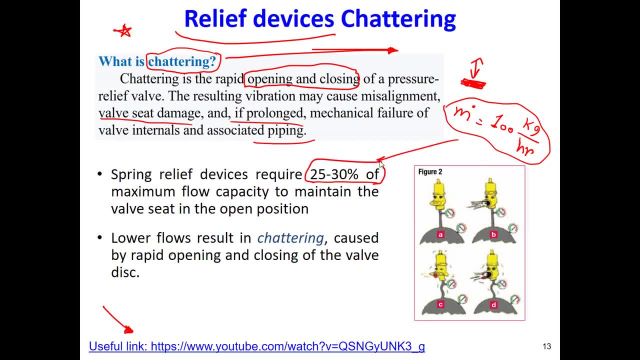 So usually 25 to 30 percent of this maximum. So usually 25 to 30 percent of this maximum Velocity or maximum capacity is needed to keep the valve open. Otherwise the valve will be- I mean the valve will be- chattering, okay. 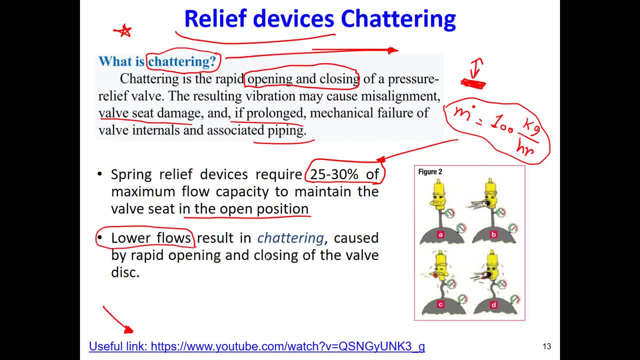 Lower flows or lower flow rates, lower velocity will lead to chattering, That is, that is an issue, and it can damage the valve. You can watch this video, It will show it. I think the better way. Okay, So chattering. 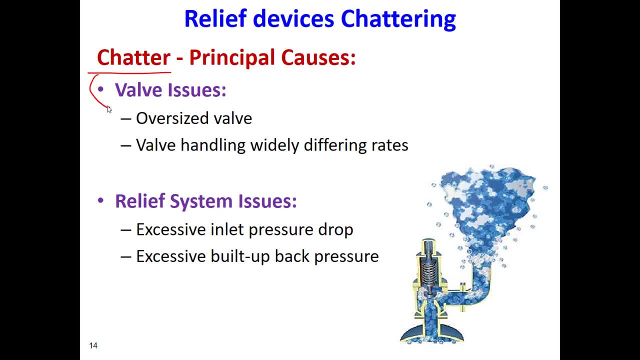 Can be again can be due to two reasons: Valve issue, the design issue and also the relief system issue. Okay, So I mean like where it is installed is wrong in a, it's inside the wrong place. So, valve issue, as I said, it can be an oversized valve. 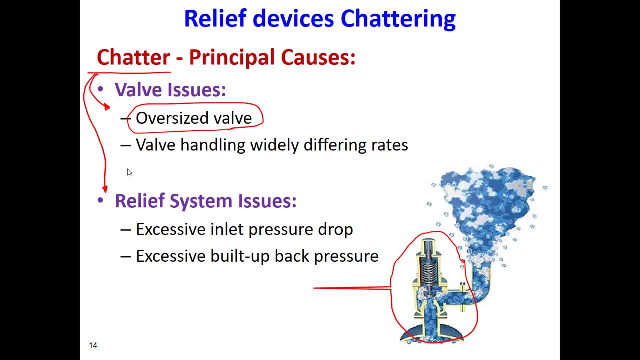 I mean, like we are using the valve, We are using a bigger size than what is needed- Mm-hmm- And valve is handling a really different flow, flow rate or different fluid. Okay, So this is, this can be the reason. 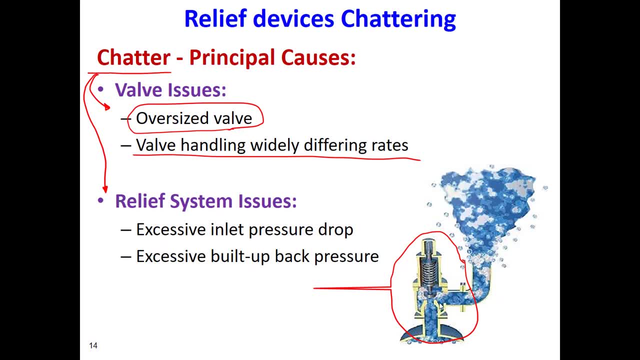 Or or the pressure here: Okay, Excessive inlet pressure drop. So if the valve again, if it's choose in the wrong way, it's handling a liquid or fluid or vapor, That is that is not. I mean like, that is that is not designed for. 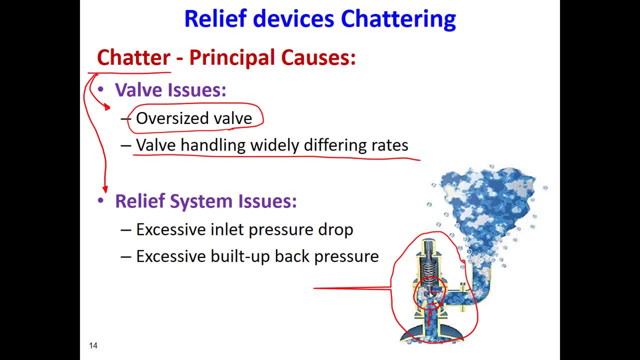 So there might be a big pressure drop in the inlet of the valve- Okay, In the in the inlet and outlet of the valve, Or if the that that will lead to chattering, Or if there is a big back pressure. 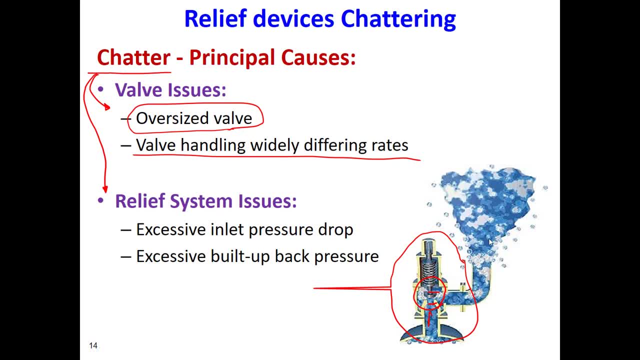 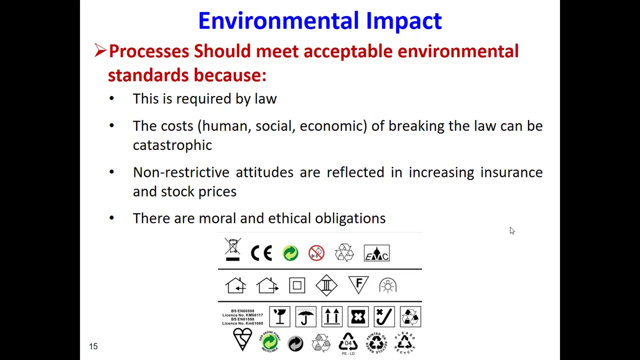 If there is a excess back pressure in the relief section of the relief valve Somewhere here, Okay, Those are also cases that we might have chattering, So we have to avoid it Then okay, That was about relieving system, which is both, I mean, which is really related to the safety of the process. 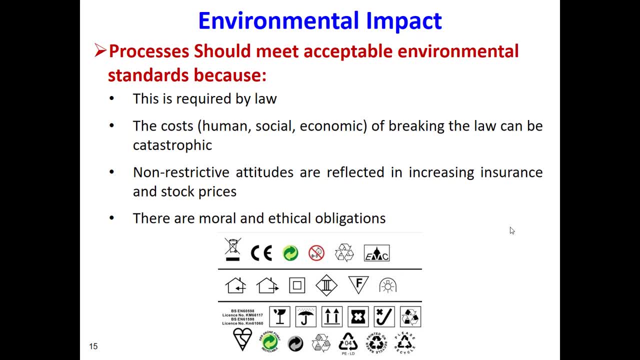 Now I'm going to talk a little bit about environmental impact of the process. So any process that we design and we are going to install, We are going to run It should be environmentally acceptable. It should be based on environmental standards, environmental regulation rules. 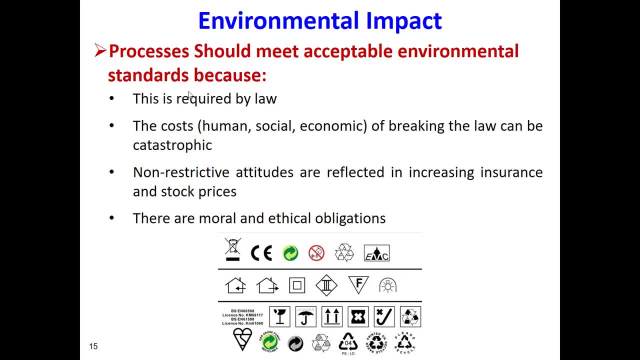 That, first of all, these rules, these environmental standards, are required by law. So I remember that in Qatar, when you are going to do tenting, When you want to have a tent somewhere Somewhere In the desert, like somewhere in the desert, like, let's say, anywhere in Qatar, that usually people they do it during the winter, or I mean during the fall. 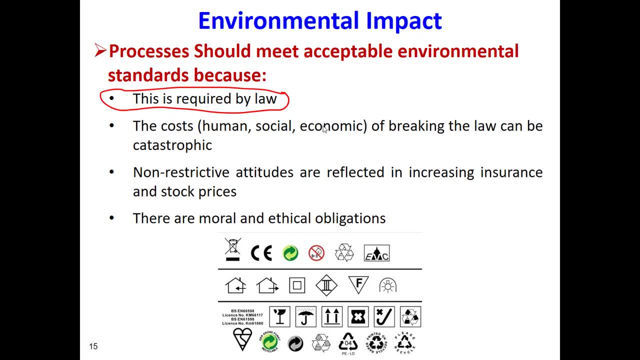 So, as I remember that some of the students they told me you need to have a permission from environmental ministry environmental office Right? So even for doing small things like that, you need a permission to make sure that you are not damaging the environment. 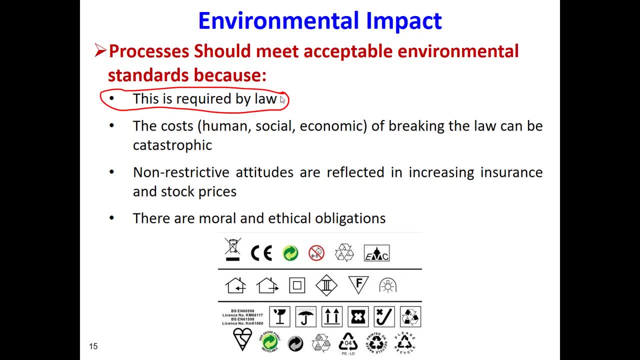 And for imagine, for a plant that is producing a lot of waste, a lot of emissions. So this permission, this kind of regulation, is even more restrictive. So the environmental- okay, the environmental standards are required by law. There are laws about that. 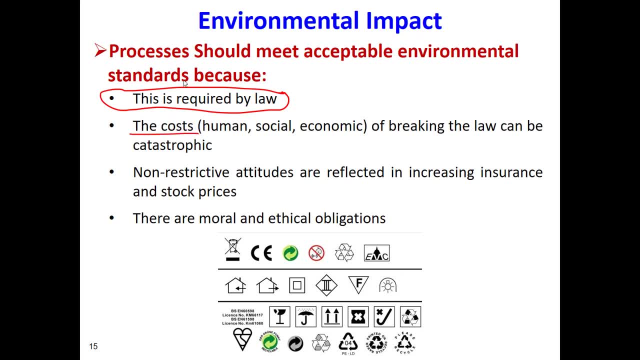 Okay. Sometimes if we break this environmental standards Or the laws, we can have a catastrophic effect on the human, social and economic, human life and society and economy. There are many examples of, you know, like catastrophic events or accidents that happen around the world. 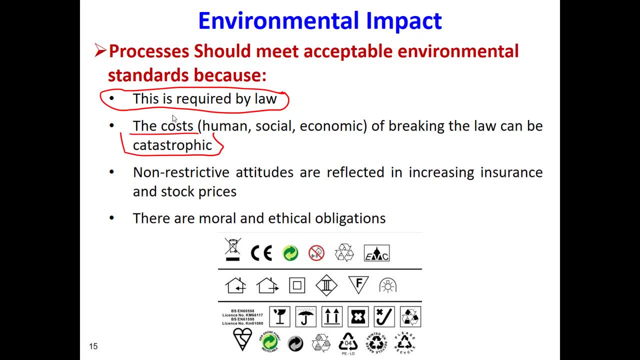 And with a huge, huge impact on the bad impacts actually on the environment. And there are many cases, There's many examples. One of them is Chernobyl. It's an atomic reactor in Chernobyl That, you know, like is like, which is like the biggest catastrophe in our center. 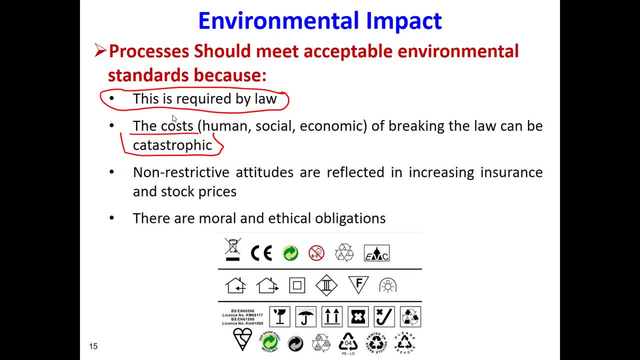 And we haven't- I mean we have not yet got any other, I mean like any bigger accident after that, That catastrophic, I mean issue with the reactor, Atomic reactor, Then okay. so then if we don't respect the environmental standards or, you know, the safety standards, what will happen? 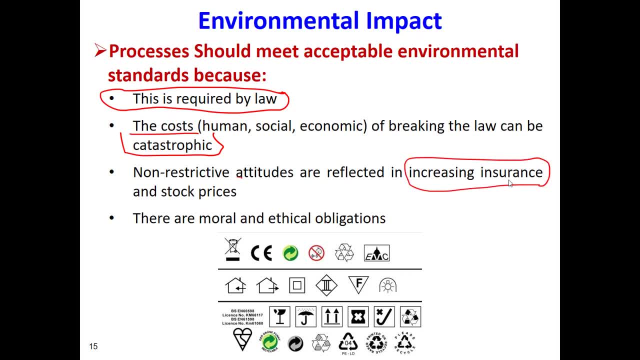 So the insurance they get more expensive. The stock market, the stock prices will also increase. That will affect the economy and the life of the people And also- this is also something related to the moral and ethical- ethical things, you know. 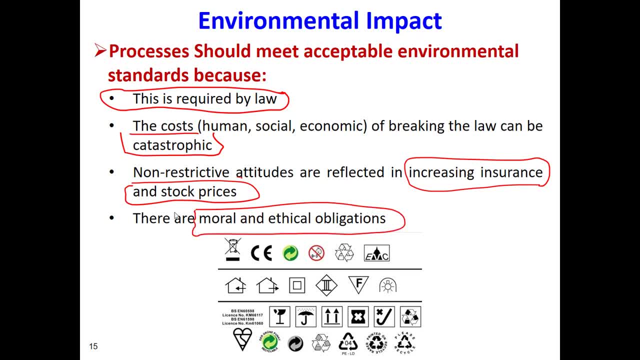 It's a moral and ethical. It's a moral and ethical obligation. We all feel some responsibility for our future generation, So we have to respect our environment. We have to, we have to, we have to respect the environment. We shouldn't damage it, because this environment is also. this should be used by the next generation, right. 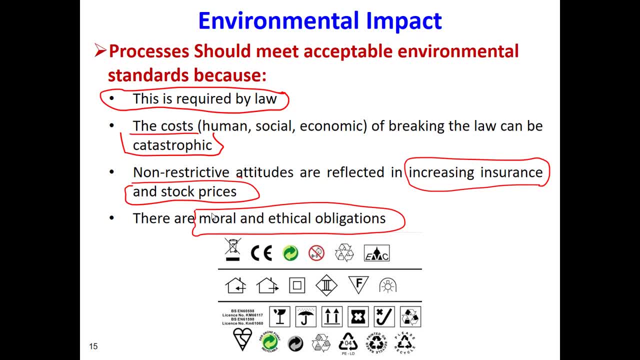 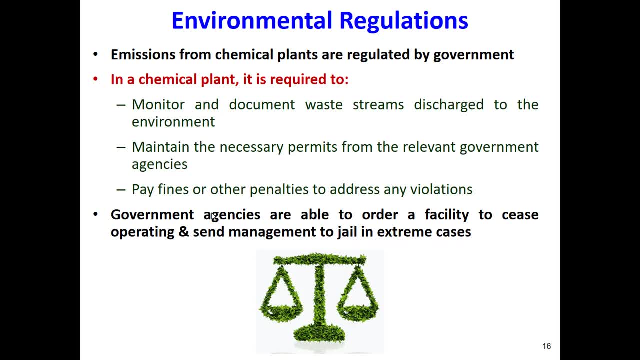 So those are the important points about the environmental impacts of the process And some considerations. Okay, there are environmental regulations either globally or locally for each country. So, like each country has his own rules- Qatar, Canada they have, or other countries around the world, they have their own regulations- 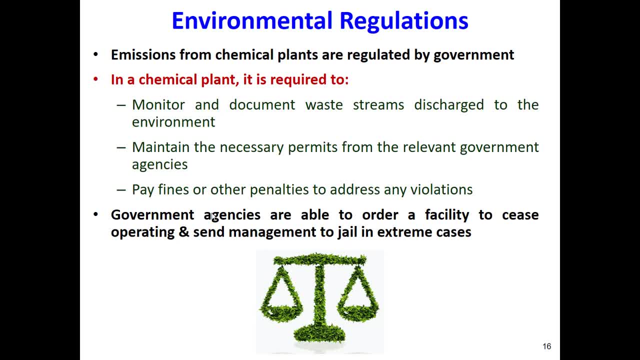 Some of them are really tough and very restrictive and very sensitive And some of them are also, you know, Like they are not that restrictive. For example, I know in Canada they're very restrict. I mean it's very restrictive. 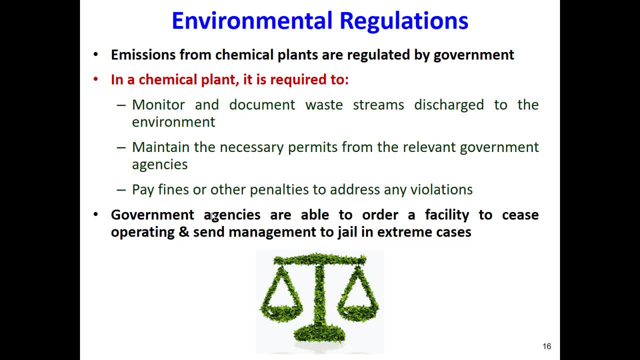 And you have to follow a lot of laws and rules to be able to do some, some kind of production activities. Okay, And most of the time okay. so the governments, they will regulate, regulate this, these things. And, for example, in a chemical plant, in the, in the chemical plant, 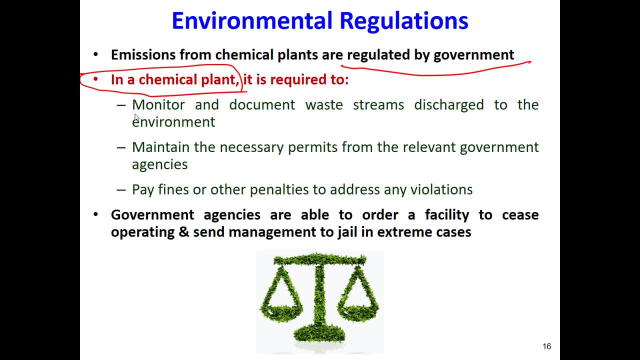 chemical engineering plant. they will regulate these things, Which is our field. So the governments, they are asking you to continuously monitor, document all the waste streams that you have And is: discharge, the environment, the contaminations, the amount of the waste, what is included in your waste. 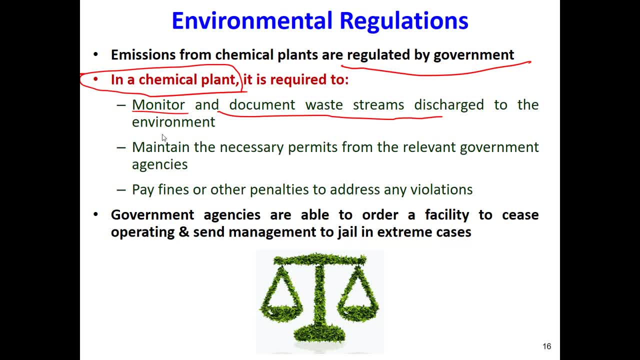 Those are, those have to be documented, monitored continuously, I mean, and systematically. Then Maintain the necessary permit. okay, so you have, for any activity that you do, you have to have the relevant governmental, the permit from the relevant government agency. 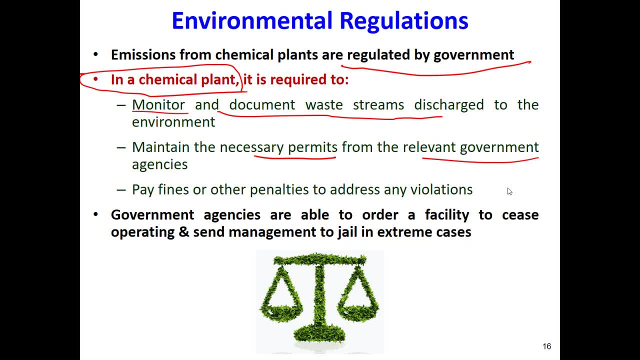 And in case, if, you, you, if, in case, if you involve in any violation in the process in your plant, you have to pay the corresponding penalties and fine. That is usually huge, huge amount of money. Okay, That most of the con companies they avoid to, to to get to any violation, to to get involved in any violation, to avoid paying such a big penalties. 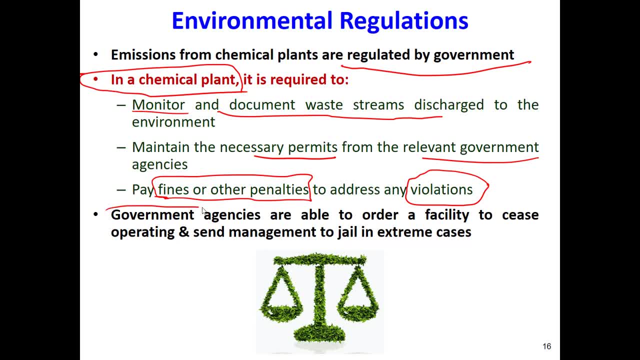 Okay, In general the government agencies, like, let's say, environmental ministries, they have that much power that they can seize operation. I mean, can they can stop operation of a plant and even send the management To the jail. 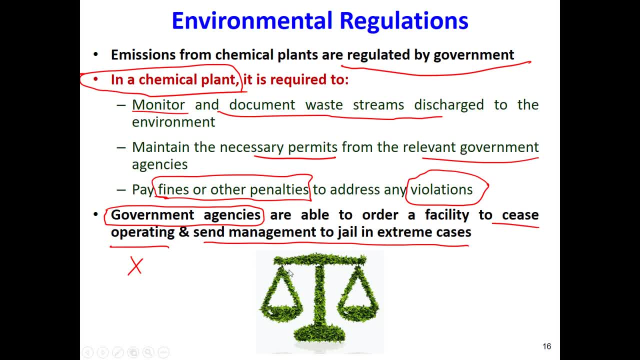 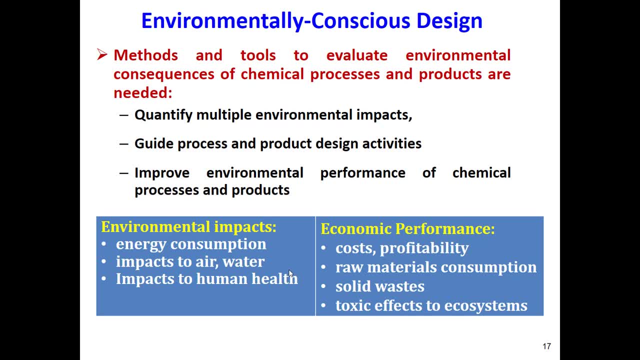 Okay. So in in the extreme case, this can also happen. Okay, Most of the time, when we are designing a plant, we will talk about environmentally conscious design, design or environmentally smart design, That is, that is, a design that we consider the all the environmental consequence. 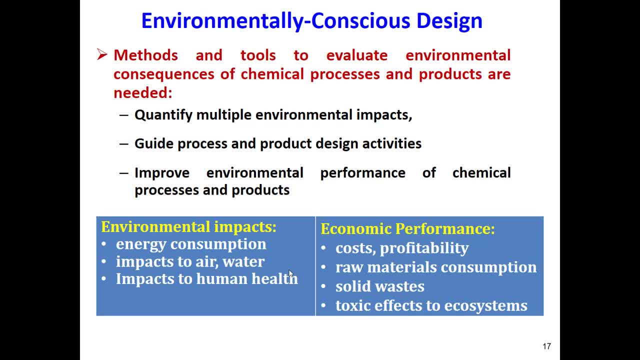 All the environmental consequence Or the design That is, that is, the design that we consider the all the environmental consequence Or the design Or the design impacts of our chemical process and product, so like to- I mean, like some of the terms that is taken into account in environmentally conscious design- is we? 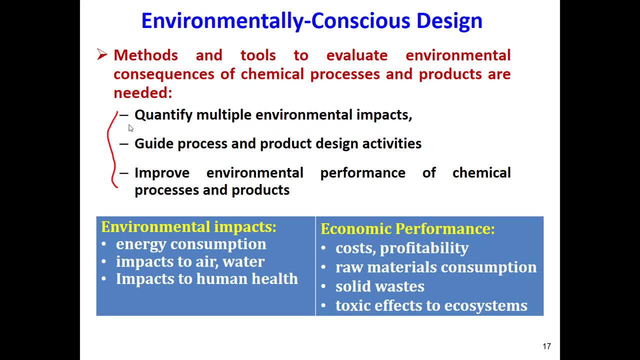 have to quantify multiple environmental impact. we have to do a lot of accurate calculation to know what is our quantitatively, what will be the impact- environmental impact, how much CO2 we are releasing, how much waste we are releasing. okay, we have to do really really accurate calculation for that and 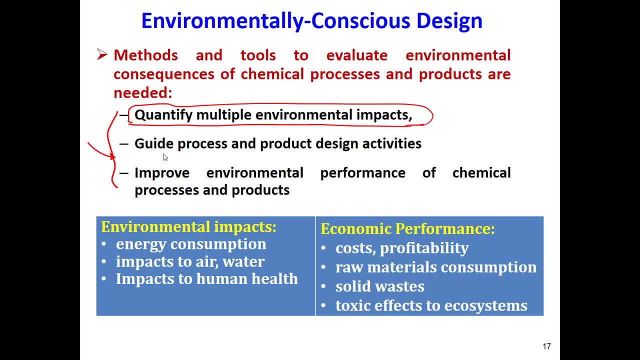 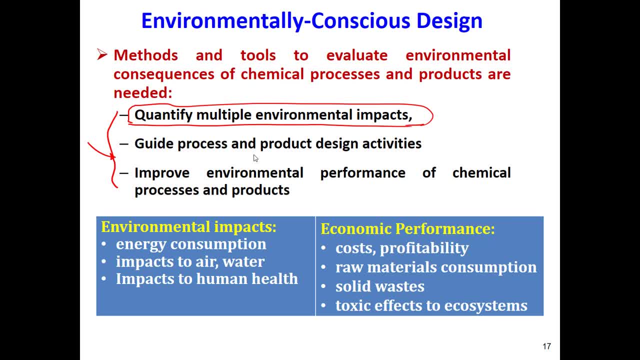 reducing some by-products than wasting. so those are the things that will be considered and also we have to always try to improve the environmental performance of our plants or chemical plant and product. those are the things that we consider in environmentally conscious design. so again, we have to you. 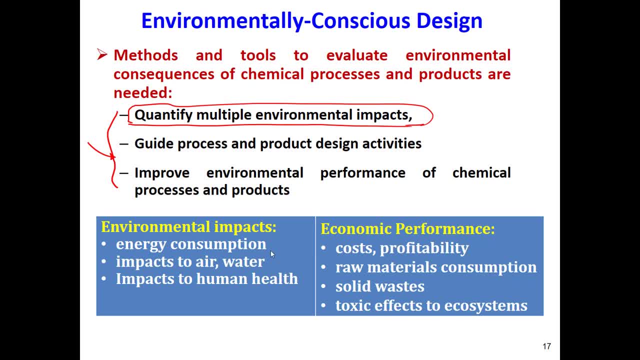 know like, consider the environmental impact and economic performance. performance I mean how much energy we consume. what will be the impact of our process to the air or water? what will be the impact of our process to human health? what's the cost of our process and how much profitability, how much raw material we are going to consume? 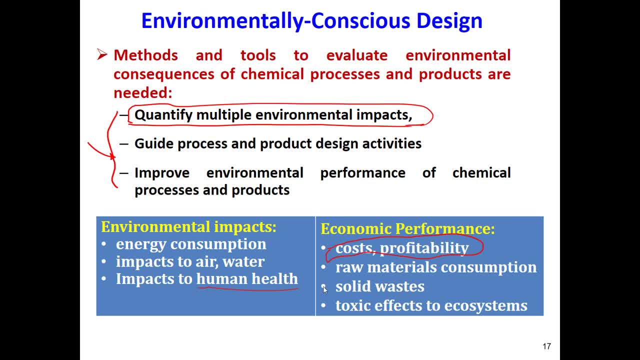 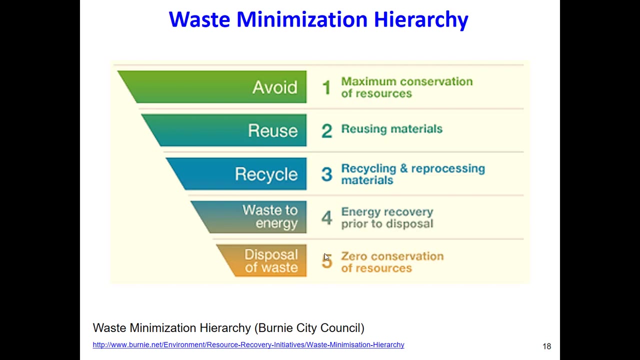 how much solid waste, liquid waste- we are going to produce and, finally, how much toxic material we are going to produce and how they will affect the ecosystem. Those are the important points that we need to consider. So there is a waste minimization hierarchy. 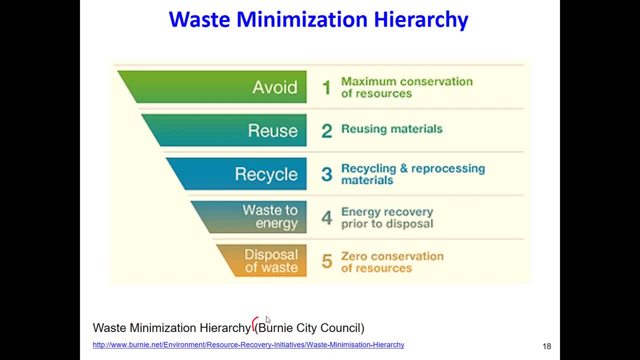 This is one example That has been designed by the Bernie City Council. but we have this type of hierarchy for different processes, different applications. Hierarchy is like you know. it kind of shows off what are the steps that we have to follow and what is the importance of that process, of those steps. 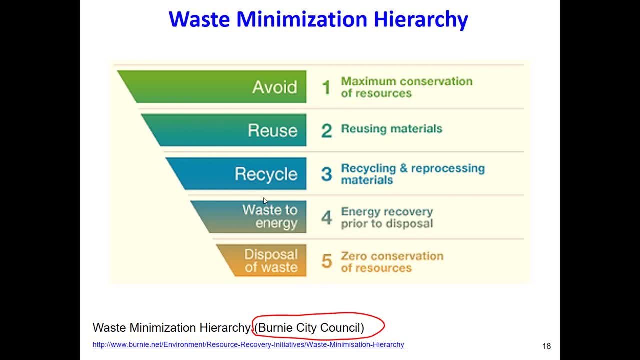 This is the general steps: Avoid, Reuse, Recycle Waste to energy. Disposal of the waste. The last thing, the first thing, important thing that we need to do, is to avoid consuming right. We have to reduce our consumption and it means maximum conservation of resources. 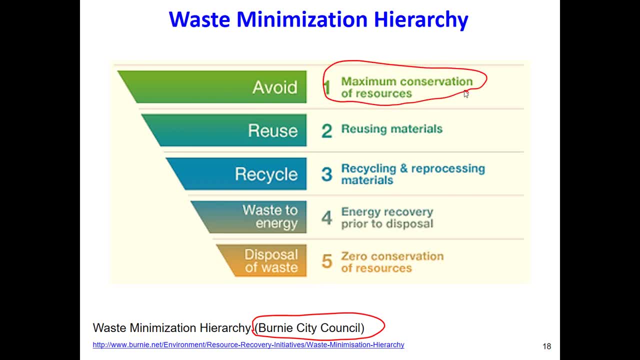 We have to conserve our resources. we have to save our resources to just use it when we really really need it. So we have to reduce our consumption. We have to save our resources. even eating, wasting food, like those, are points that we can do it personally, that 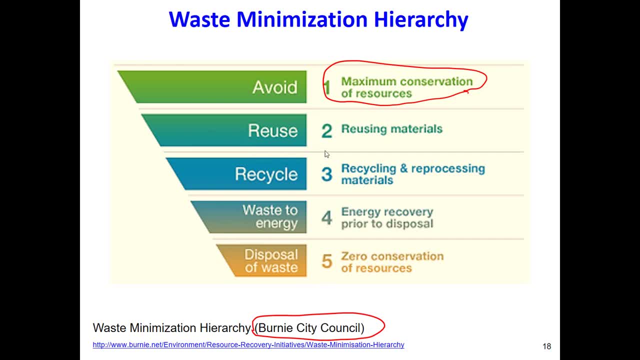 will affect the whole whole universe. reuse, okay. so there are many matter: the arts that we can reuse them, right so dark cars that we can use them for many years, done. there are devices that say laptops, many products we can, cell phones, we can use them for many years. we, just we, or if let's say we don't need them. 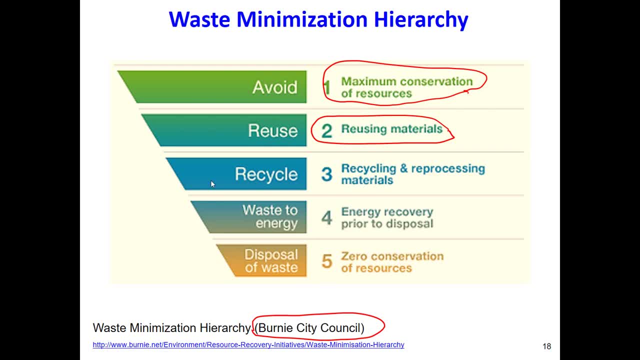 today we don't need to waste them, we can just keep them. maybe tomorrow, you know, day after- we can reuse them, recycle if we really need to base something. so it's better to recycle it if we really don't need laptop- not nowadays. they are, like you know, the company that they recycle electronic devices. they 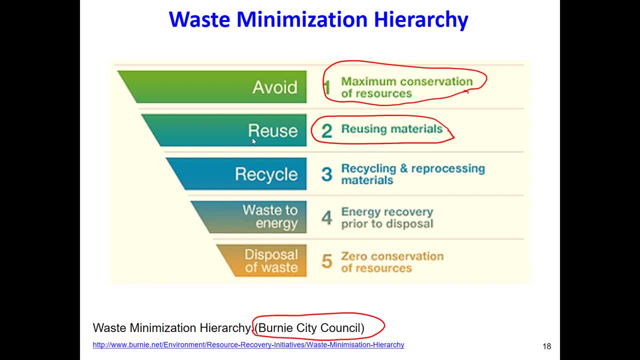 divide the recycle cell phones lab size. why? because each laptop, each electronic device, it contains plastic materials. it can right, so you can see easily you can do it with any kind of devices. it can be right, so you can see easily you can do it with any kind of devices, it can be. 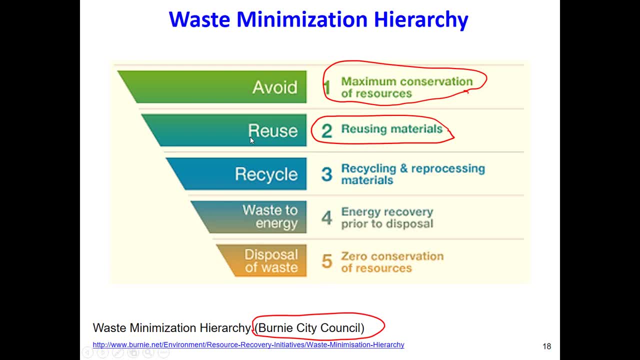 in content. that's a different type of metal, like copper- you know, very expensive metals actually. so those companies, they receive this waste- waste, let's say, electronics- and they will separate different parts and they recycle them. they recycle and reuse the copper, recycle the polymers, plastic materials and almost- uh, i mean big magic- big parts of the, the electronic will be recycled. 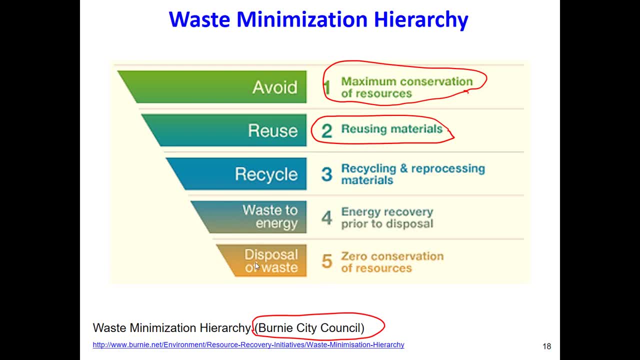 waste to energy. if you are going, if you really have to waste something, instead of sending it like that to the environment, just living in the environment, just you can. most of the time you can convert it to energy. like waste to energy is a big, big industry these days that let's say we can. 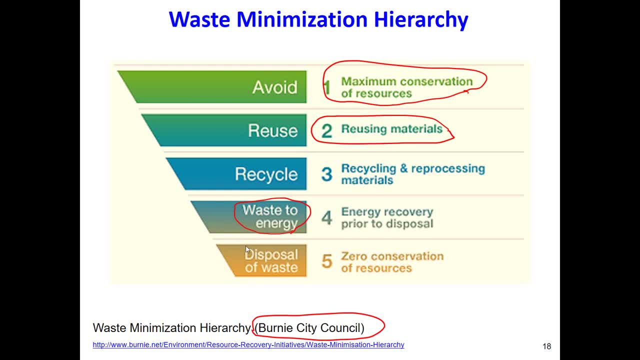 produce some chemicals, value-added chemicals or even energy by using the waste and, at the end, the last step is really disposal. uh, to the disposal, to the environment. if we really cannot do anything about that thing, that waste, if we cannot, you know, reuse it, recycle it or convert. 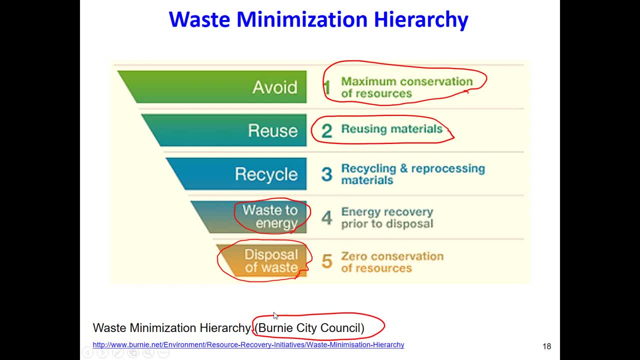 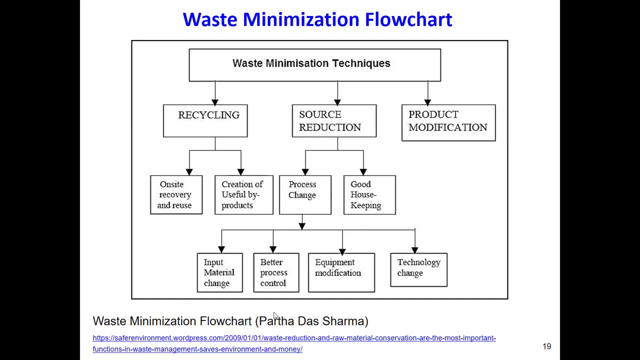 it to energy we will, we will dispose of. so this is, uh, one example. there are many other examples in the internet. you can just search it then. okay, there is another example here and it can be historic links, because maybe it costs 100 billion dollars, is too expensive to do a full year and can be think of an anonymous or downstairs. 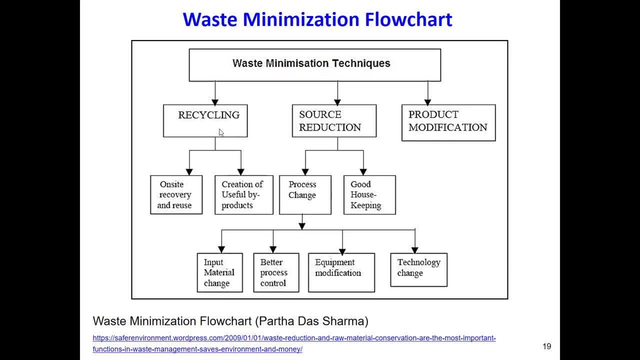 just for me, uh, just doing like the review and the uh dziejo business outside of american companies having modeling chemistry already, and the other ones like saving water and專, received all advantages reusing. those are the things that they will see. what are the potential of that process or that? 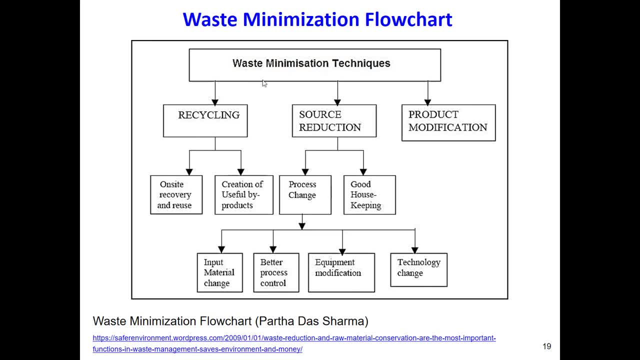 equipment to apply each of this item. so, in general, waste minimization technologies can i mean contain the three major work: recycling, source reduction, okay, using less raw material or less resources. recycling is a very important step, by the way. then product modification, modifying our product to be used for a long, longer time or do the same job with a higher performance, you know, with the 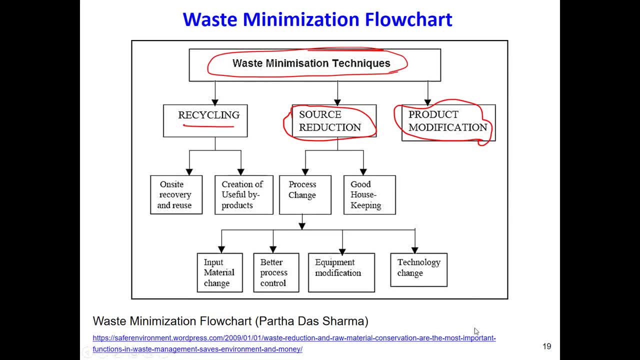 higher i mean, i mean i mean with a better quality, then okay. recycling, it can be unsightly. recovery and reuse. we can, let's say, use separators, separate some chemicals, send it back to the reactor and reuse them and recycle them. or if you are producing some waste, we can clean the waste, we can treat the. 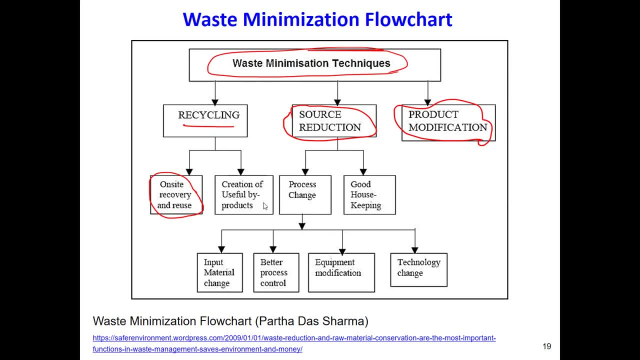 waste and reuse it in the system or, let's say, producing some by-products. okay, before wasting that component, that chemicals, we can convert them to some by-products this will have- this is happening in many processes- source reduction to reduce the consumption of the resources or raw material. what we can do, we can. 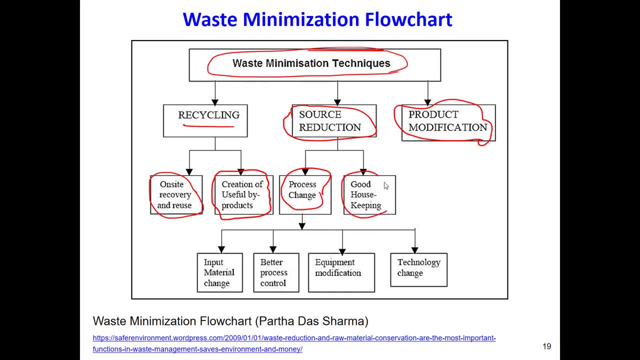 change our process, modify our process. good housekeeping i mean, or maintenance. this also help us to reduce the use of our material. then, okay, process change again. it can be changing the input material. okay, we can change once again for a longer period of time. i mean in the process. i mean is not change. 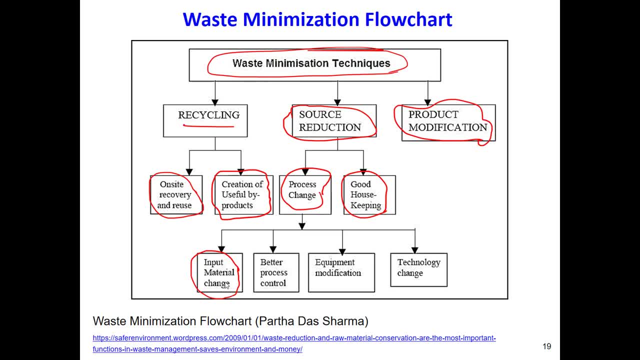 the material. we can make them more pure by using some separation process, or even we use the material that is best fit to our process. better process control: if we can control the processes more accurately, more precisely, so this will also lead to a better quality, product quality, less waste, less pollution. 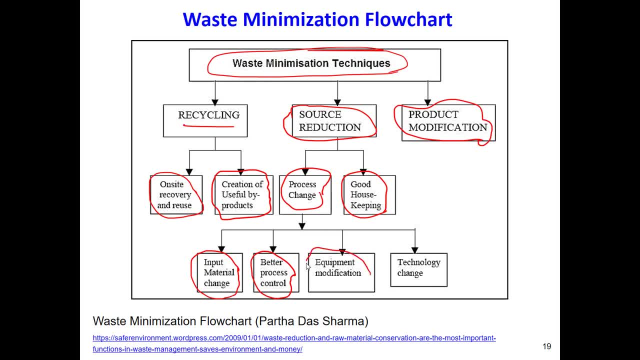 emission equipment modification. we can change the design of the equipment and this will be also connected to the better control, and I mean process control and technology change. sometimes, you know, we can also change the technology, let's say, for treating the waste. sometimes we can use. we can use. 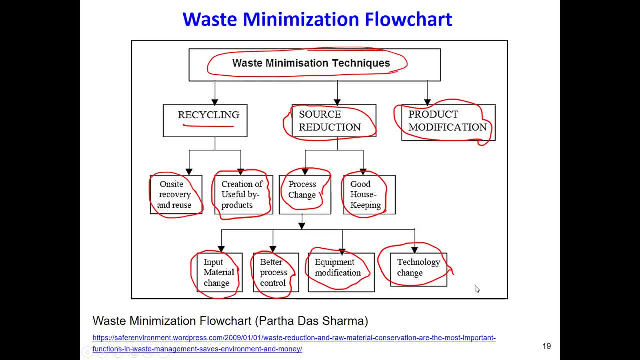 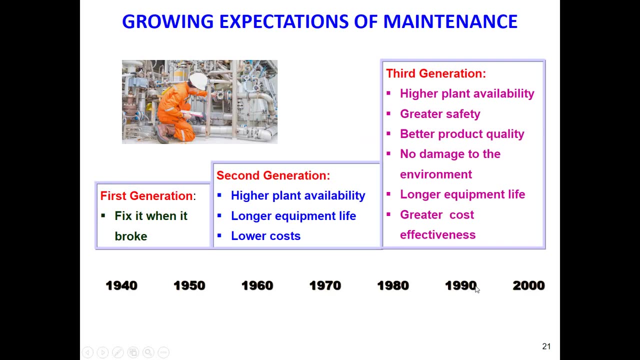 fermentation, we can use combustion, we can use gasification. those are the process technologies available. so that's kind of gives you some idea about how to minimize the, the waste. so maintenance is a very important activity in the process. if we do it right- maintenance, good maintenance- we can save a lot of money. we can produce a very I 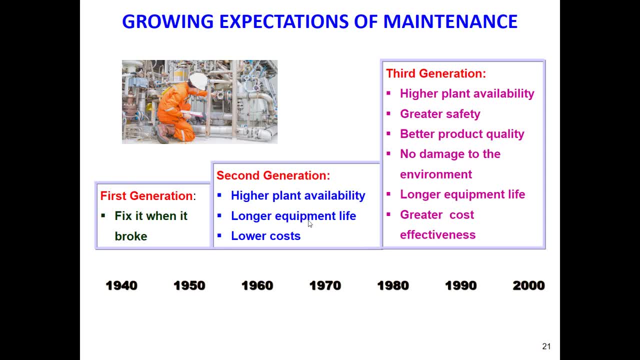 mean higher, better quality products. that is in the benefit and we can, I mean, avoid producing waste. maintenance: you know there have been a big development in the process maintenance, let's say since 50 years, 70 years ago, up to now, okay, 60, 70 years ago. 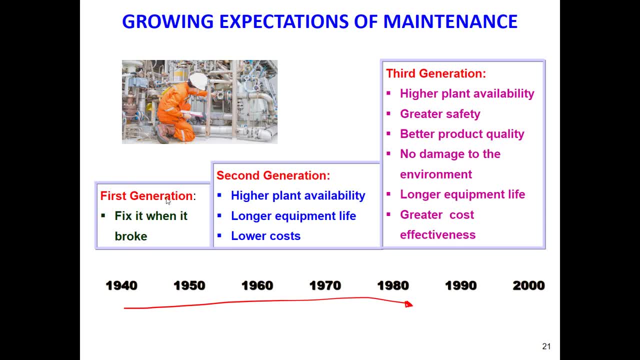 up to now. so, like they are saying that, in general, there are three generation of maintenance works, okay, so the maintenance activity, which is also a process, which is also a, you know, like each company, they have a group, they have a team. that is a maintenance team, okay, and they have a really. i mean, they have a. 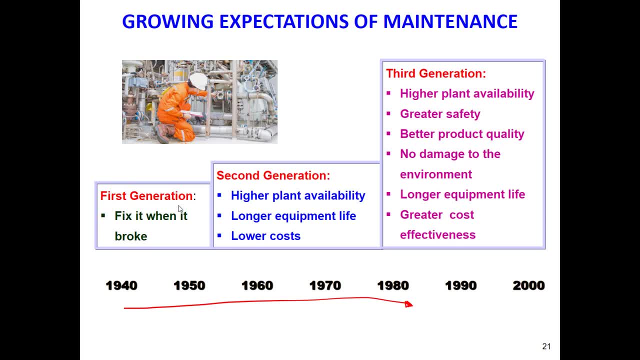 very good protocol to follow and to to do the maintenance activity. but i mean, like many years ago up when, you know, the industrial revolution just started, so the maintenance was not very, you know like, was not taking very seriously. but uh, okay is on, uh is uh okay. so there have been a lot of development. so before i mean like those early years, that 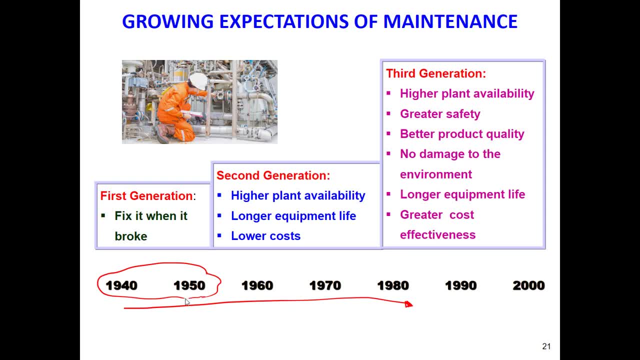 you know, we had kind of industrial revolution. most of the plants they just start to producing, you know, per dogs. so it was the maintenance was just fixed. when it's broken, okay, they were waiting to see. if something is broken, it's not working. they were fixing it many years after 20, for 30 years after. 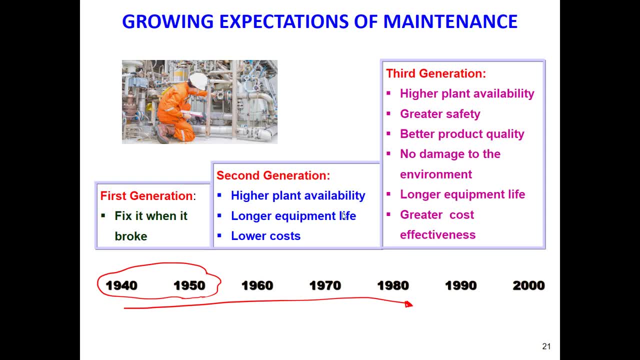 it becomes more detailed. okay, so they wanted to have higher planned available availability. they wanted to plan to work- i mean, more continuously. they didn't want to stop the process and they wanted to have to use the equipment for a long time, longer time. they wanted to have a longer life for the 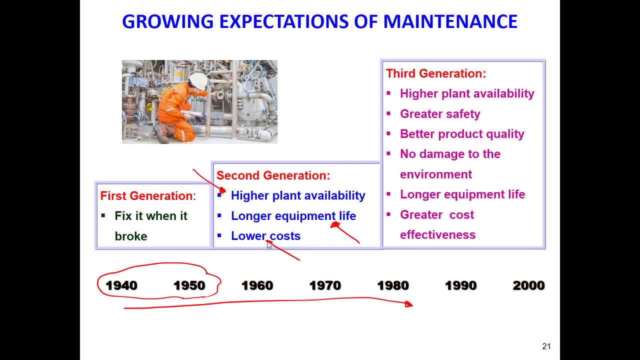 equipment and they wanted to pay less cost. so they they prepare the maintenance activities based on these objectives, and after that i mean the recent years, in the last 20, 30 years. so the maintenance has been much more uh, accurate and it's been like a bigger activity that contained 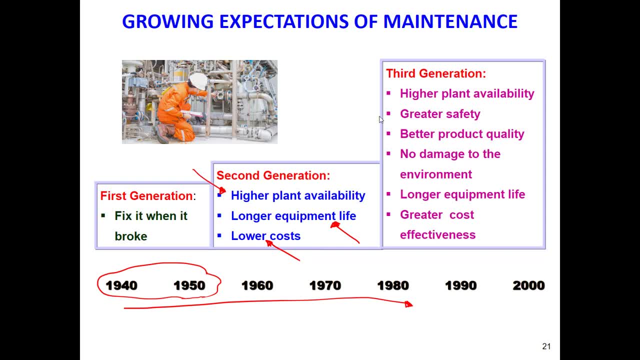 that is aimed to reach to a higher I will- availability, better safety, better product quality, no damage to environment, longer equipment life and also the less cost or more more profit. okay, so those are the things that is being considered. that is being considered when I mean for the maintenance activity in the recent year. 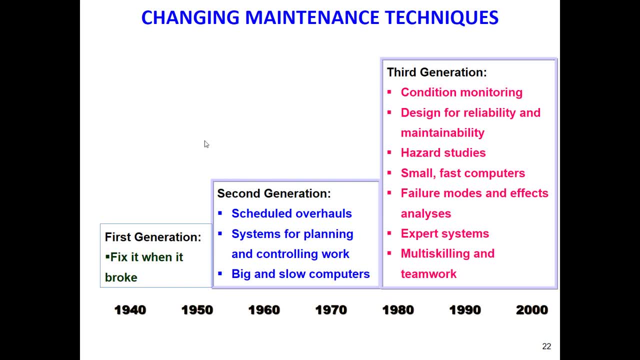 and okay. so the techniques, the technology that was used, okay, that has been used for this job has also changed. we had okay, so before it was just fix it, then in the first generation, fix it when it's broken in the second generation. you know they were some systematical and a schedule overall. 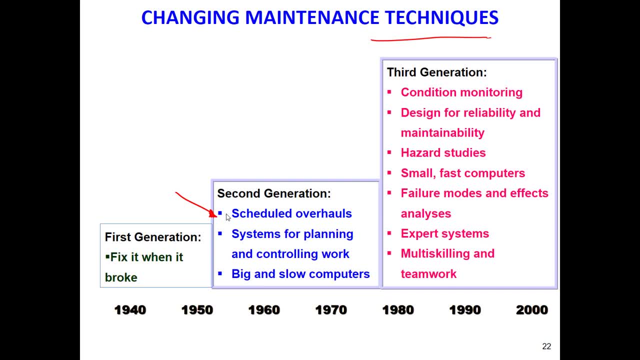 you know they were some systematical and a schedule overall means, you know, like, let's say, they were stopping the heat exchanger after each few months and they were cleaning, fixing it and then putting, put it, putting, putting it back in the operation. so that was the schedule overhaul system for planning. 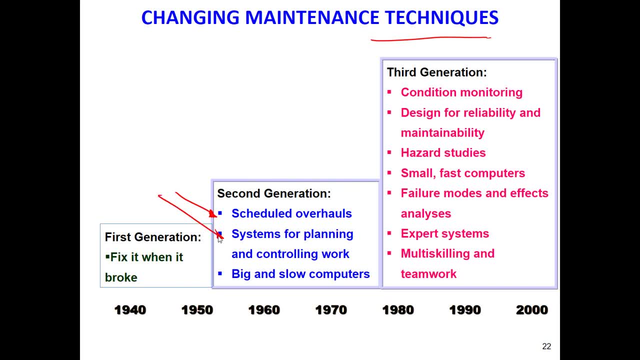 and controlling work. so like they had a work, you know like the systematic workflow planning work and you know, like for maintenance and also like computers- that was those times that they were big and slow- they also help for this maintenance thing. you know the scheduling, the maintenance. but third generation okay. so in the third generation we had more. 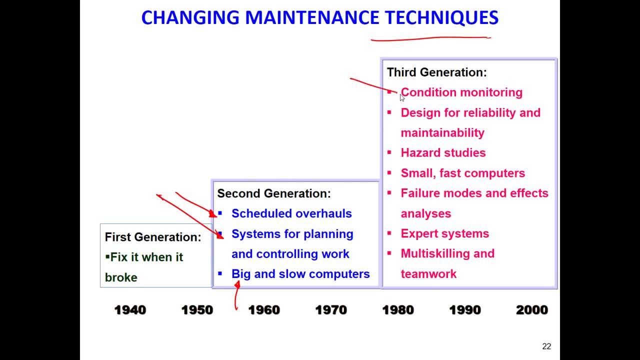 more technology, more instrument that we could monitor the condition of the equipment. really there were many technologies, softwares that you could design. you know the main 10, the maintenance walls, and there have been many hazard studies and this days we have very fast and small computers that 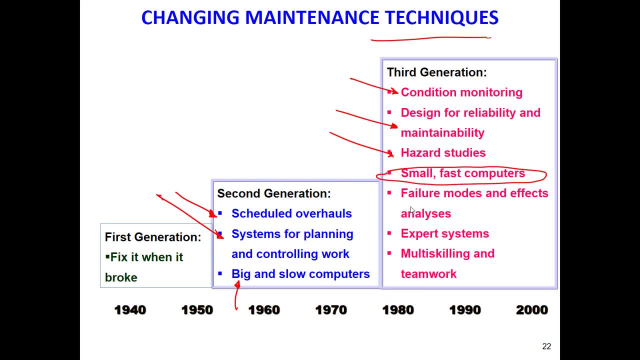 can be used and there are many, you know. analysis like for for failure mode and face, you know, like a lot of simulation about that, a lot of expert systems. you know there are a lot of people that are expert in this job, at this. they, they have been. 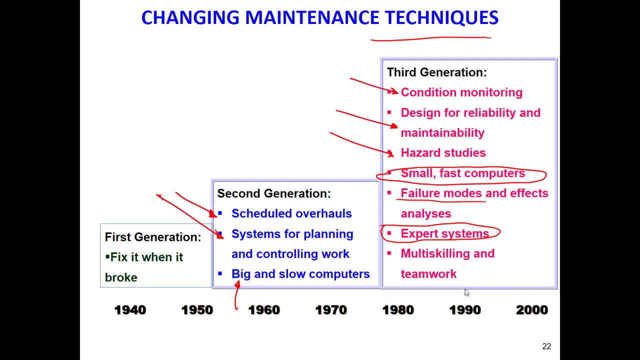 design and maintain the maintenance works and there have been many hazard in different you know and institutes, and also multi-skilling and teamwork, you know like. teamwork is also encouraged because maintenance is something that most of the workers they have to be involved and collaborative to do it. 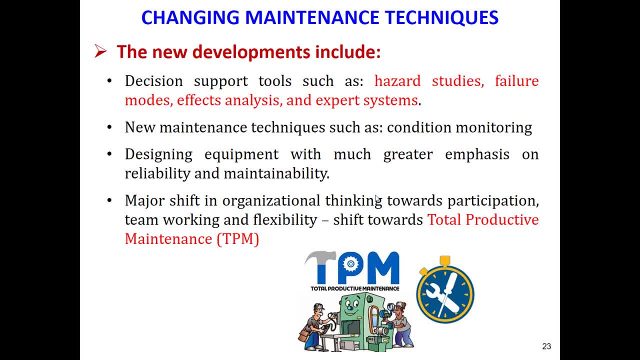 carefully. okay, so the new development or the new new development or a new methods or technologies for for maintenance is aim for total productive maintenance, TPM or total productive maintenance, so that is considered to use tools for hazard studies for the failure and effect mood and the failure mood analysis we are 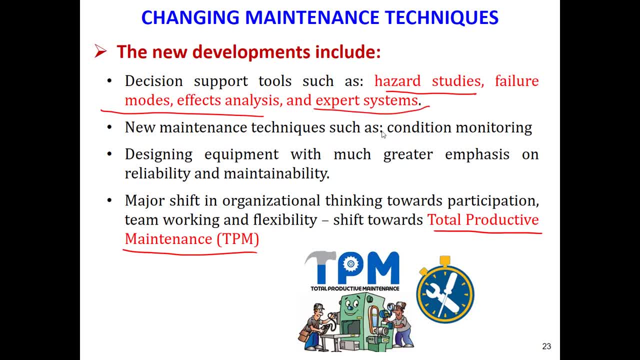 applying the expert systems. condition monitoring is also new technology or new methods that you can monitor the condition of your equipment. it is in the good condition but condition it is working, is its maximum capacity or there is some issues? so you can really monitor. you don't have to wait until the equipment fail and then 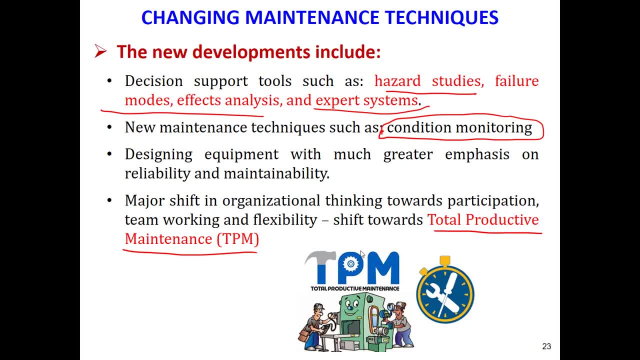 take some action, you can really monitor the condition of that equipment. nowadays we have more technologies for fabrication, for construction, so we can design and build equipment with the better accuracy, with the more emphasize on reliability and maintenance and ability. so that's another thing, that for the design equipment and also there has been a major shift from individual 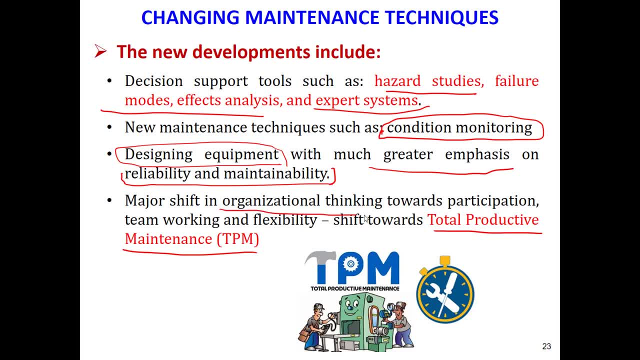 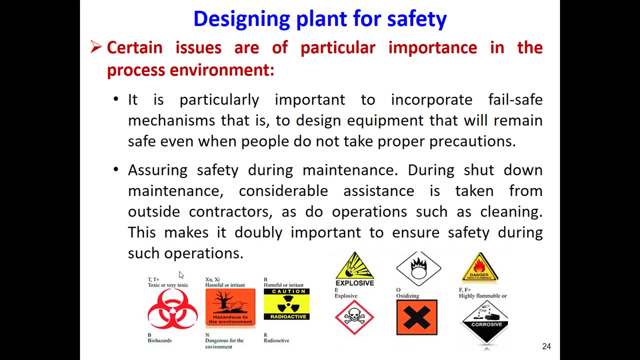 working or thinking to organizational thinking. okay, organizational thinking by in, by power, by, you know, like encouraging the participation, team working and being flexible. that is all of this activities is aimed to lead the total productive maintenance, or TPM. okay, so about also designing? so designing the plant is also muy. 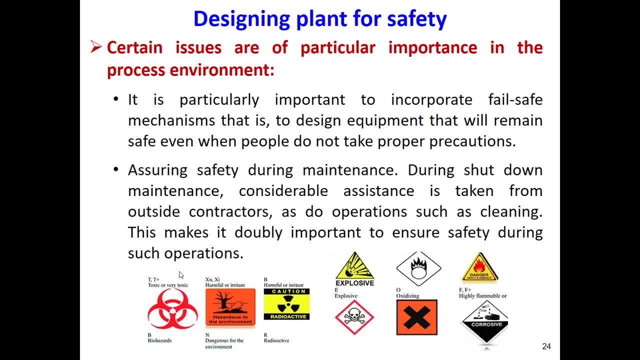 know, when we are designing the plan, the design equipment, there is one, one phrase that is saying that designing plan for safety. you know, it's very important that even if the in the plant there are some equipment that they fail, or if there is a maintenance work is going on, so the plant is a still safe, okay. so there you. 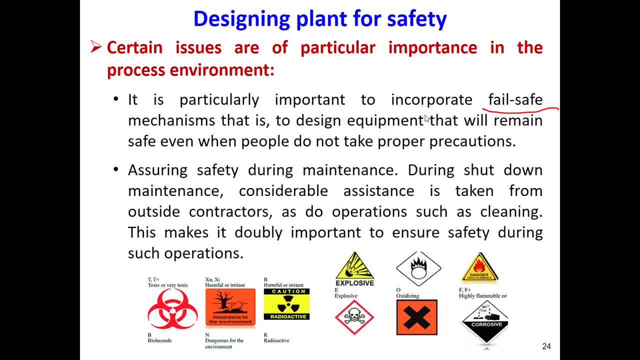 might hear this term fail-safe. okay, fail-safe mechanism is that the equipment, it has been designed in the way that, even if it's failed, the process will be a still safe, the equipment will be a still safe. that, as I said, one of the example how we can make sure a fail-safe mechanism, let's say designing some. 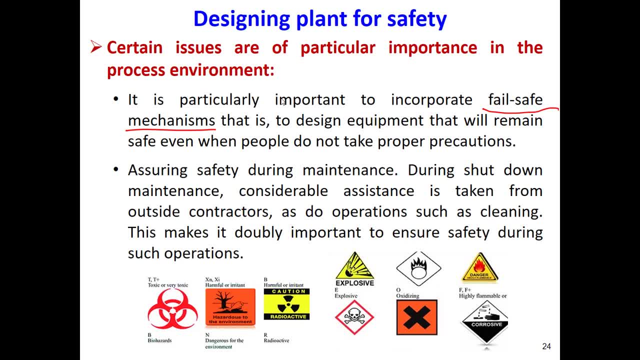 switch, emergency valve, some pressure with the relief system, this kind of system they are, help us to reach to such a such a mechanism. then during the maintenance- okay, when there is a shutdown for maintenance- we have to also make sure that the process is safe to do the maintenance. let's say sometimes you have, you have the 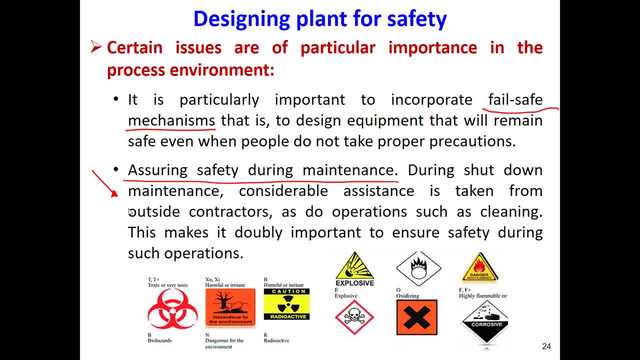 equipment that you need to clean it. so you will commission that to outside. you will, you will bring a contractor from outside, like a company that is expert in cleaning, to clean that equipment. so you have to make sure that the process is safe for them to come and do the. 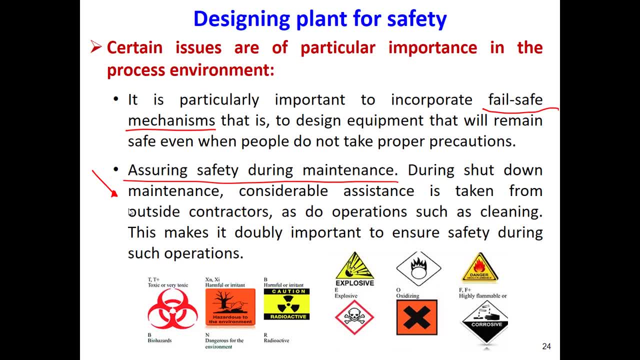 cleaning, the maintenance work is also being done safely. okay, so like there are many cases of you know, like really the catastrophe, catastrophic accidents that let's say, they stop one equipment and they start doing the maintenance. they didn't think really what will be the effect of that and stopping that. 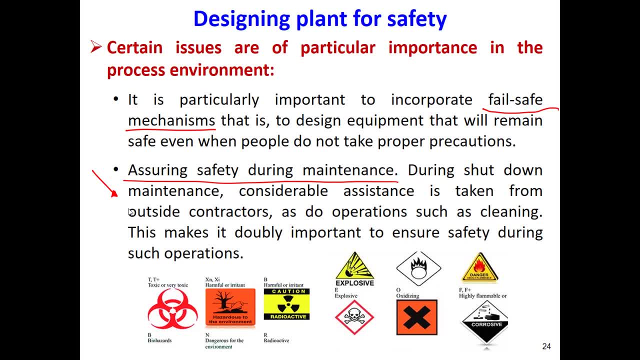 equipment or that maintenance to the other part of the plant that that led to really, you know, like explosion or you know cut to a very bad accident. it there are many cases, you know. if you just search in internet, YouTube, you might, you might find, you know, those cases. not like in aviation industry, you know, for the 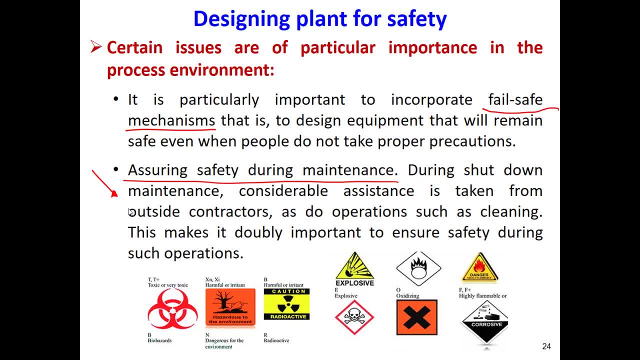 maintenance. maintenance is a very important part and whenever the maintenance is done on the aircraft, usually when they land, there is a protocol to maintain the to check many things in the aircraft. so, like once they they do the maintenance, the overall, they have to submit a very accurate, precise. 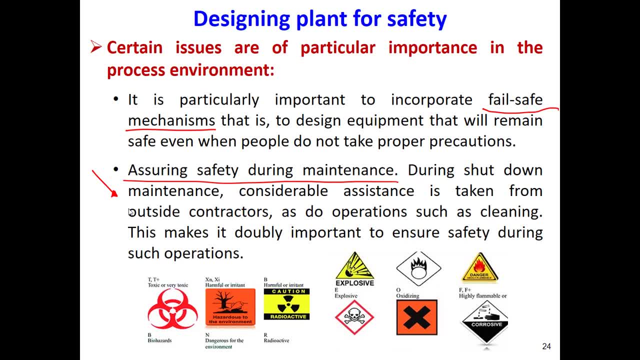 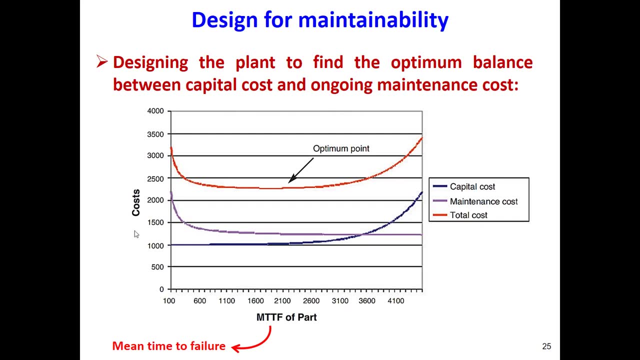 report to the managers, to, or the pilot, so to make sure that the aircraft is safe to to, to, to take off or, you know, to work again. so those are some points that we need to consider. okay, so then, when it comes to the maintenance, maintainability, I mean like: 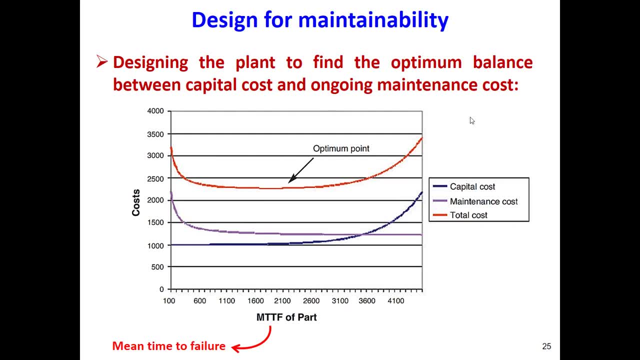 one question is always: what's the optimum age of of equipment or a part to be used in the process? okay, there are to do that, the op, to find the optimum age of a part. okay, equipment in the process. there is always such a curve like that that can be used by the designer, by the managers, to make some decision. what is? 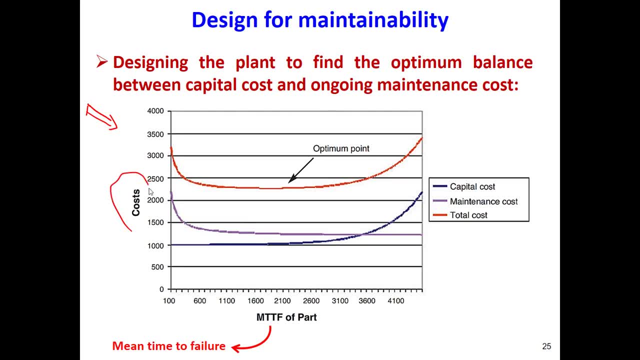 this curve. so you have in the y-axis you have cost. in the x-axis you have mttf of the part of equipment. what is mttf is mean time to fail. so it can be, let's say, days- usually is days, it can be days, it can be weeks, it can be years. so you have mean. 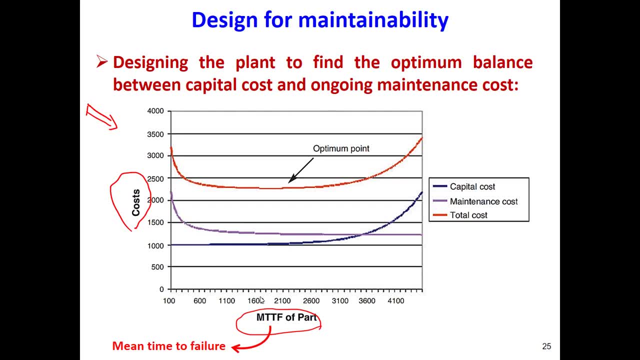 time to fail. this is the time that that I comment that part. we will check. so for that part the capital cost, usually at early age, early days, early years is is is not increasing because, let's say, inflation is concern. so you, you buy that part, that equipment, you will install it, so you don't pay really any money until. 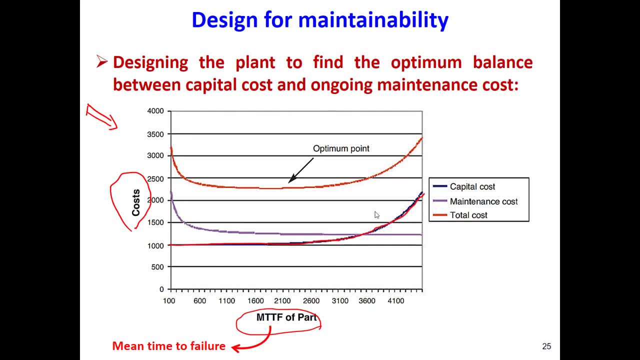 that part is good enough. start to. you know, let's say, if it's a compressor, so you need to repair the compressor continuously, you need to change the part, you need to do a lot of mean, you need to change the parts of that compressor or something you need to. 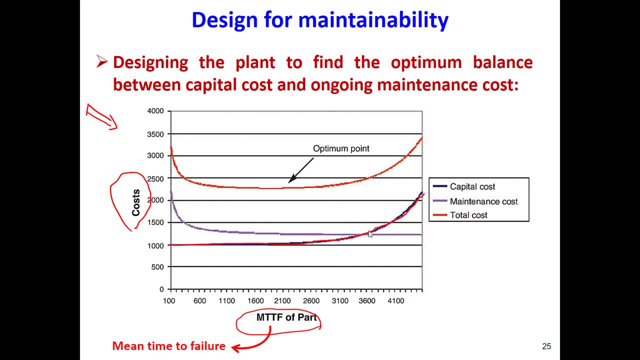 change the motor, the driver, the shaft so that increase your- I mean that increase your- your cost of that equipment. once it's, you know you start using it, after few months, few years it will start to become costly for use, like a machine, like a car that gets old. it has more money to change. you know you have to. 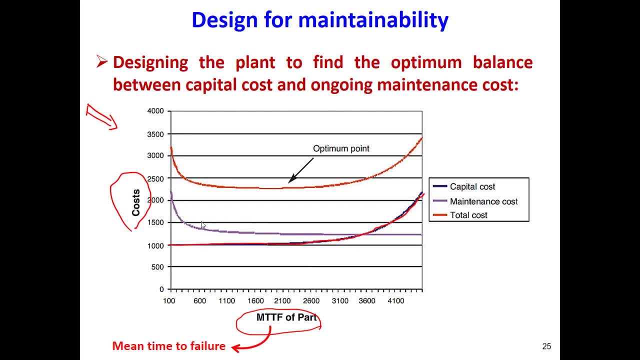 change different parts. you have to change the, you have to change, you know, the tire, this kind of thing. that is really usually capital maintenance. so the equipments you know once are in assault at the beginning, they need a good maintenance, you know like, because you need to need to change in the beginning, they need good maintenance. you know like. 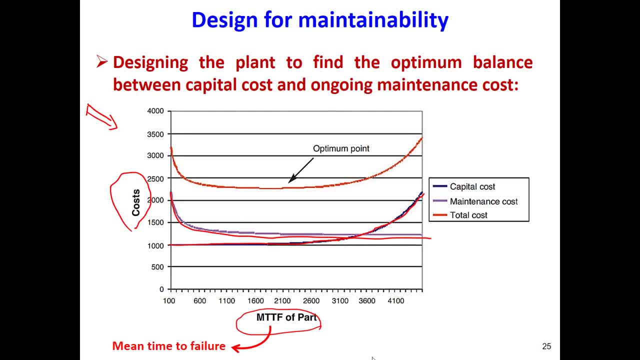 to fix a lot of things you need to, you know, like change the oil, let's say continuously. you need to make there is no leakage, continue. so at the beginning it has some kind of maintenance cost and but as long as it you know like it start working, the maintenance cost will be less. 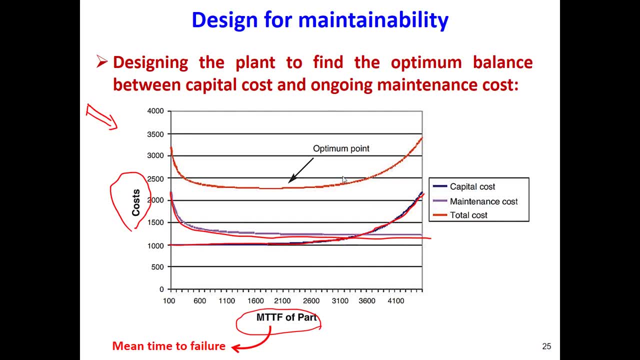 but capital cost mall might increase. there is a point, there is a age, there is a range that this total cost- total cost, which is the of the maintenance and capital cost- will be minimized like, let's say, this range: that is a minimum total cost. so is this, this range? tell us the best, is the? 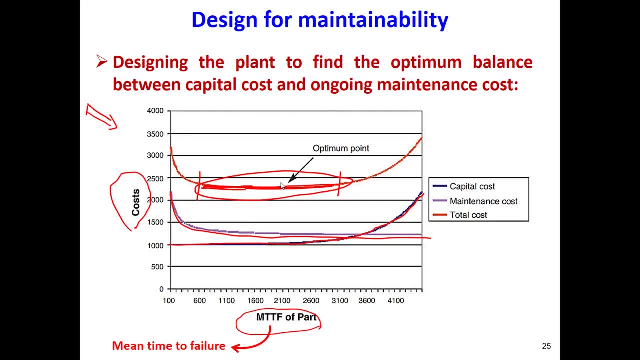 range that we can use that equipment or that part in the best way is the best time of range, range of time that that equipment or that part can be used. out of this one, you can see that the total cost will be more. so we have usually such a such a curves, such a graph, such a tools to be used for. 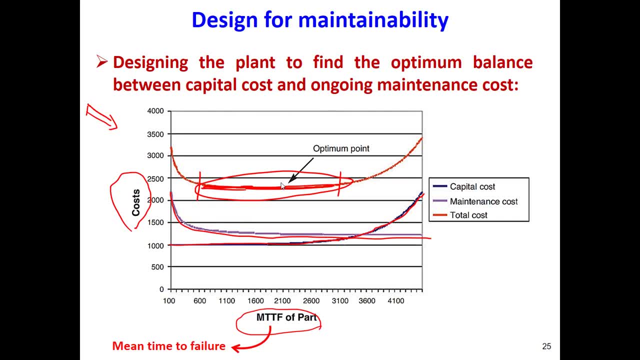 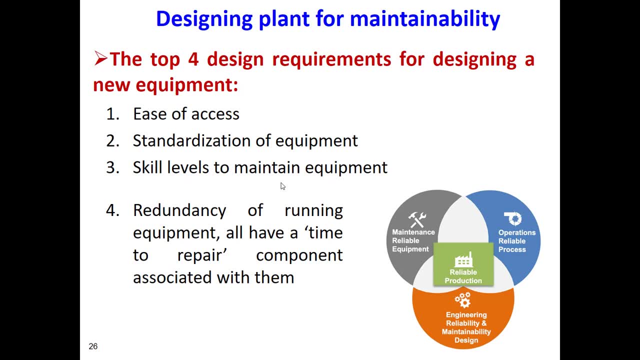 for maintenance job, and i mean evaluating the maintenance and the cost of the equipment. okay, designing the plan for the maintainability. so when we are designing a plan there is kind of four design requirements for the maintainability. for the mentality, there is four requirements. first, easy to access. each equipment should be easily accessible. we should be able to have to access. 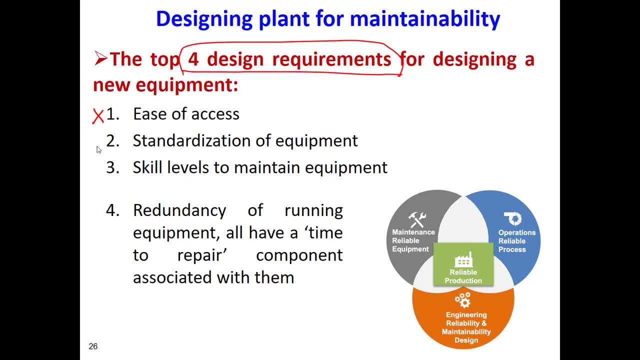 to them easily, to repair them, to change them, to replace them. a standardization of equipment. so all the equipments they have to be work working in the standard condition, the standard design condition. we have to evaluate what is the skill level that is needed to maintain that equipment. 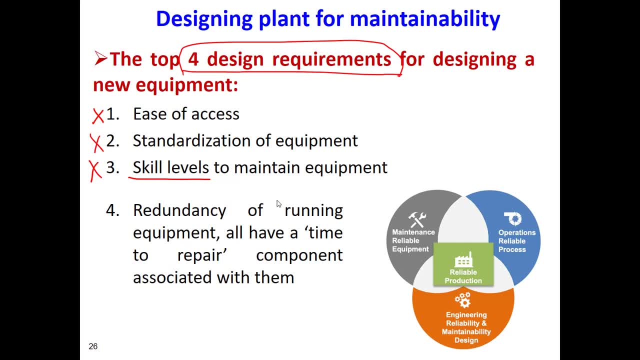 okay, this also, we need to evaluate this, we need to report this, and also redundancy of running equipment. okay, so we have to, we have to evaluate, uh like, after how many months or after how many years we can we expect to repair or replace that equipment. okay, so those are the four important things that we have to consider when we are designing the 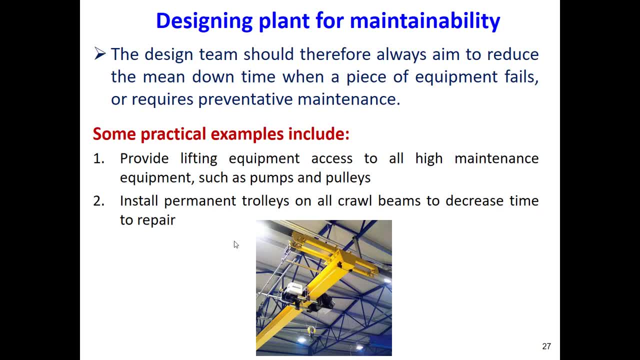 equipment. okay, one example, uh, like one example, for example, for example. so, first of all, we have to always, uh, we have to minimize the time that the equipment will fail. we have to try to design or choose the equipment that will will be used for the maintenance of the equipment. so we have to. 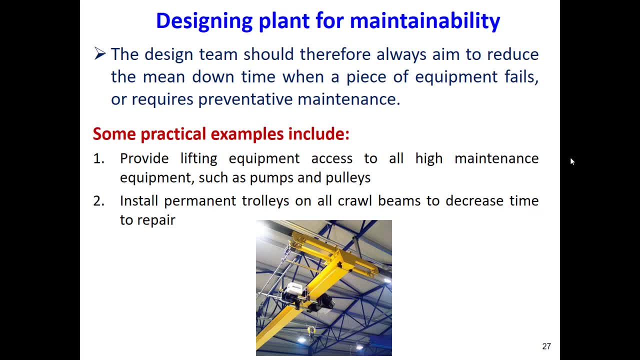 be failing. i mean the minimum way. i mean like minimum time. i mean, let's say, minimum time per year or per month. okay, so equipment has to be designed to work continuously and to be reliable. so we have: we need minimum maintenance, need minimum cost for maintenance and 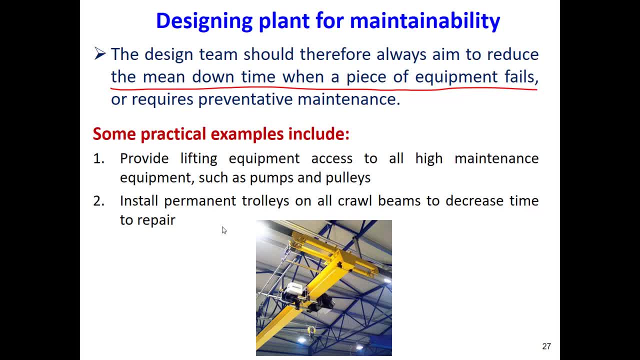 okay. some example is, let's say, for example, for pump compressor, those are the equipment that they need. they continuously need maintenance heat exchanger, so we need to. for example, for accessibility, we need to design such a lifting. you know devices close to that equipment, you know we have to make sure that. 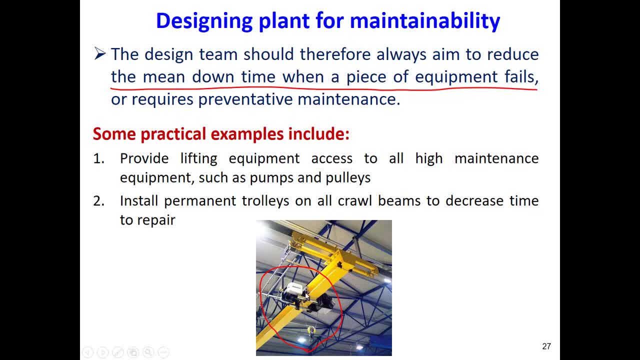 we have kind of, uh, you know, like we have already planned and installed some instruments, some devices that we can use to move that equipment. we can lift that equipment, put somewhere else, bring another new equipment replace it, do the repair. so those are the things that need to be. 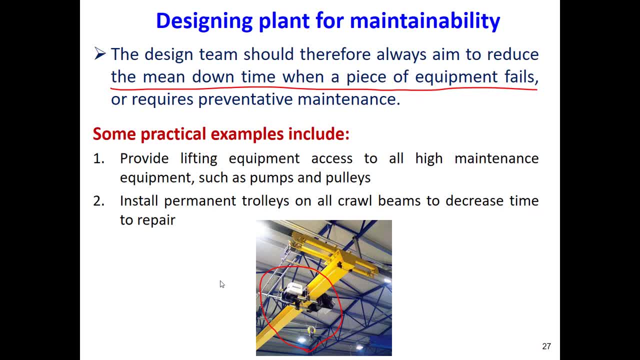 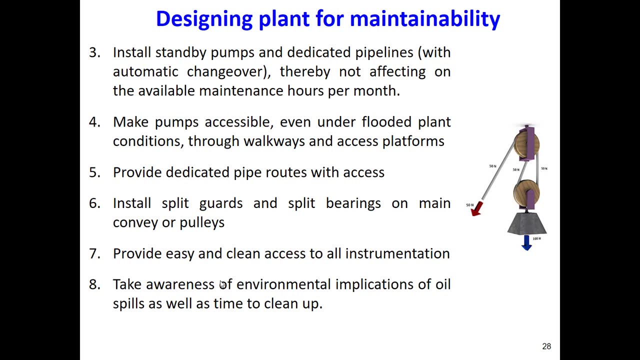 considered when we are, we are designing the plant. you know those are the details. that has to be really considered carefully then. okay, those are also some additional, additional points about designing a process for maintaining maintainability, for maintenance. so we have to, as i said for the, for the pumps. 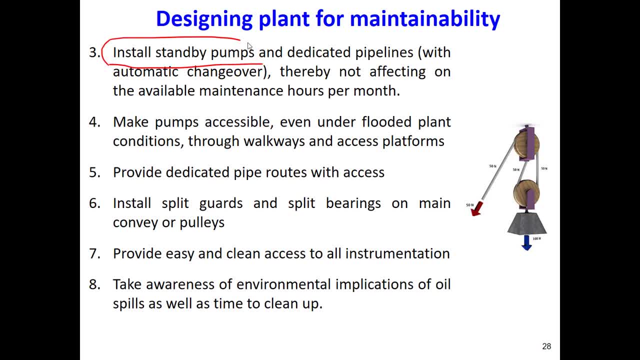 for the compressors we have to always in style standby equipment, let's say most of the time for the pumps. we also install one parallel pump or one parallel compressor. so when the problem in maintenance we switch to the, to the, to the other pump, to the parallel pump. so we do the maintenance. we fix it and then we can ruining the comparison fault. so i Unterstützung this. uh uh, what is itkehr? so we have to at some with a pair of error. so we have to, uh uh, a UMOM Opel, which is, uh, a motor side. 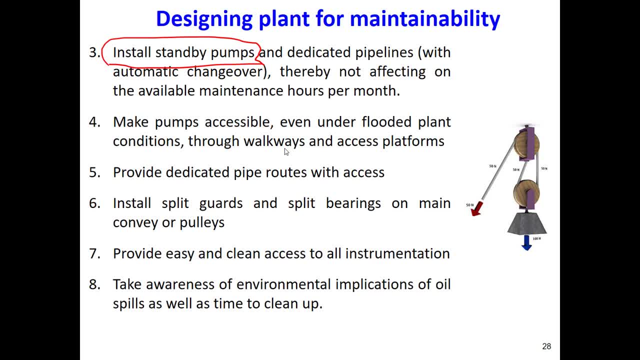 as well as one parallel electricity. so so to the other side. so we have to also have, uh uh, a water switch. back to the main part. so we need to design such a, such a things in the process, and even the pipeline, you know, we have to dedicate some pipeline that is used for purging, for 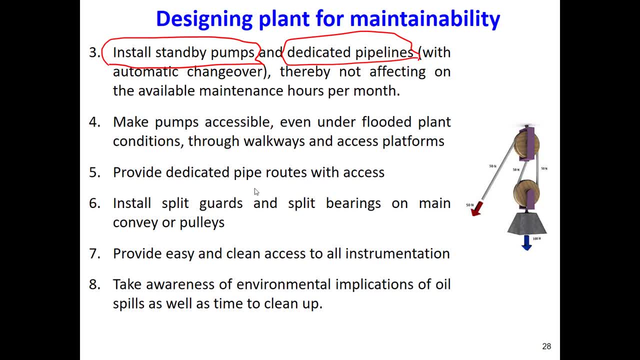 maintenance for, uh, you know this kind of work then, uh, you know, as i said, we should do, design device, i mean lifting device, moving devices to move the equipment to lift them. you know like to. we have to relocate them to be accessible. uh, those are the things that has to be. 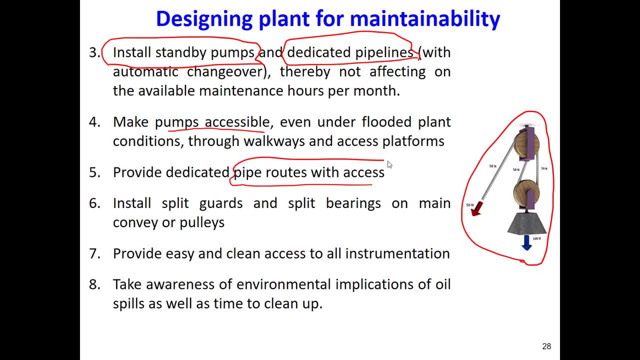 we, we should have access to the pipeline easily, to the valves, to the equipment. uh, okay, those are some. you know some additional information you can? so all the instruments, uh, the contour instruments, everything has to be accessible. we should be able to have access to them to check them, to replace them. 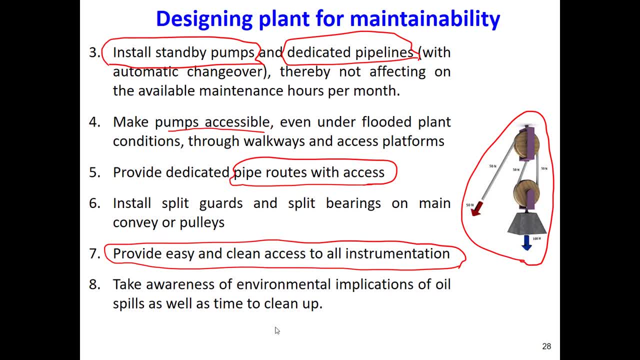 and also okay. so we have to also consider the environmental impacts of maintenance. let's say, when you are cleaning something, when you are cleaning a compressor valve or a pump that was, uh, operating with the taxes material, when you open that valve, when you open that equipment, there might be a 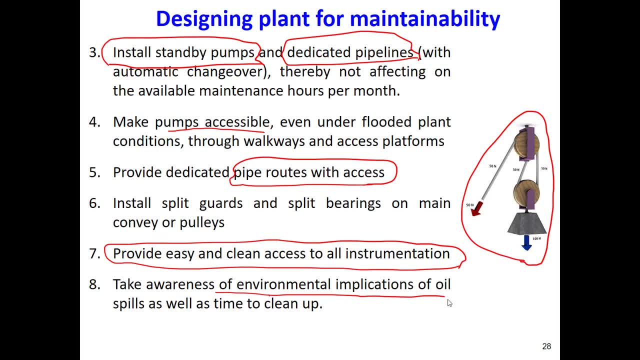 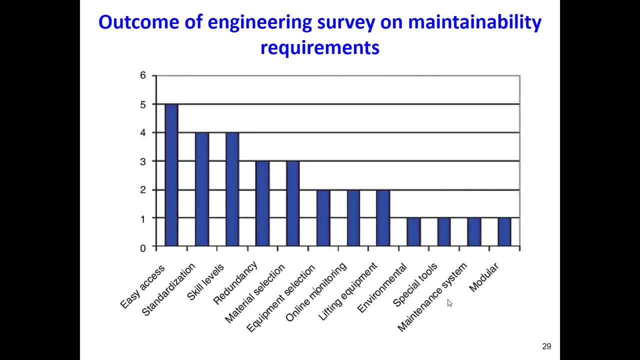 spills of those toxic materials, or you know, on the floor or you know it might contaminate the working environment also. we have to consider those things when we are going to do the maintenance. then last slide of this unit is about okay, like we have also always for the maintenance requirement. 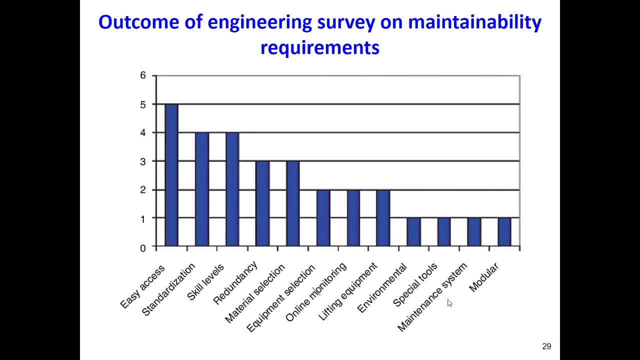 there are such curves or such figures. that is usually prepared by the maintenance team or, if either even by the design team, prior to the design and installation. you know, like it can be, how easy or how difficult it is. you know, like we give different degrees of- i mean difficulty or degree of, i mean like we give, you know the level of. 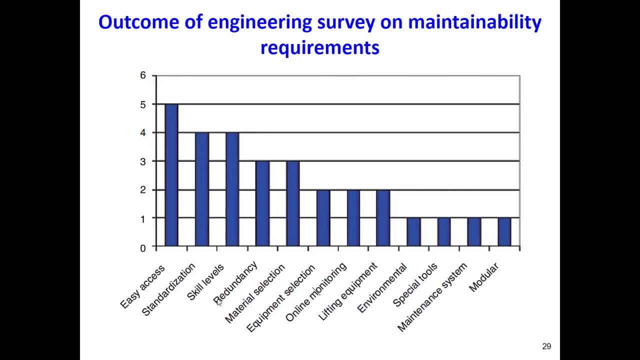 easiness or difficulty to different jobs that has to be done for maintenance. let's say we need to know how easy is access to have access to the equipment. if this is a standard, standard, standardized, standardized- sorry, a standard- dies the equipment. what's the level of skill that we need to maintain that that equipment? how often or after how long of? 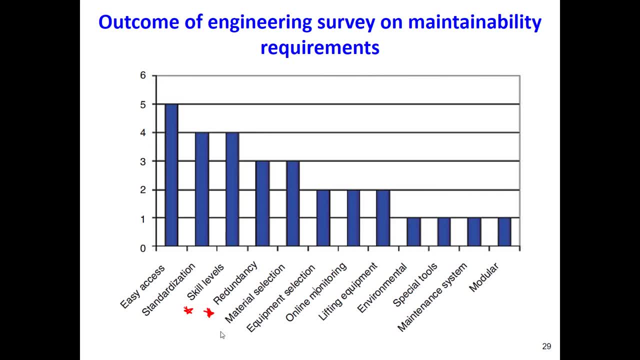 usage it will fail. the material that is used is expensive or is cheap. okay, selection of the equipment: online monitoring potential, lifting equipment that is needed, the environmental impact, some special tools to repair it and the maintenance system that is needed. So those are the things that will be all considered for maintenance requirements. 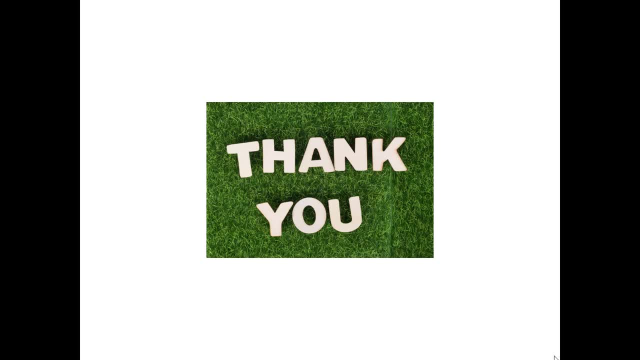 So that's all about this unit. hopefully you enjoy it. So please go through this video and try to understand all the topics very well, and I will be always happy to answer your questions. Take care and I will upload the video for unit 9 soon, next week. 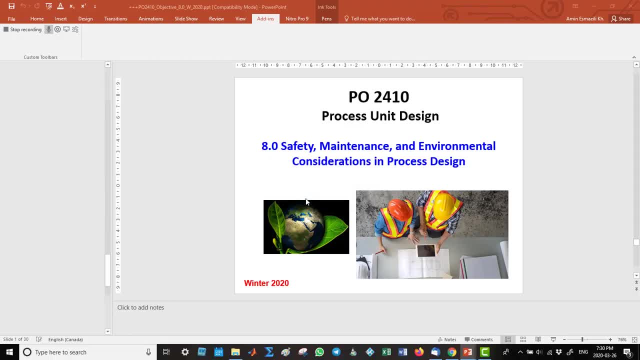 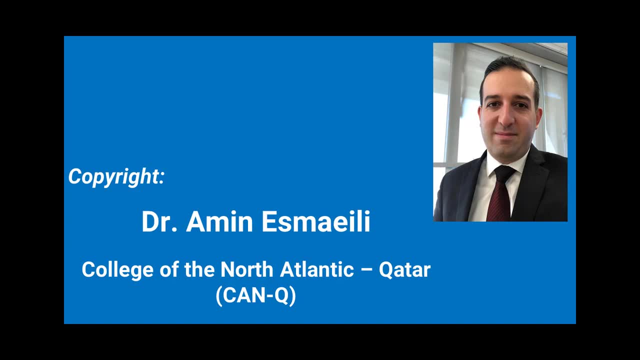 Thank you. Subtitles by the Amaraorg community.